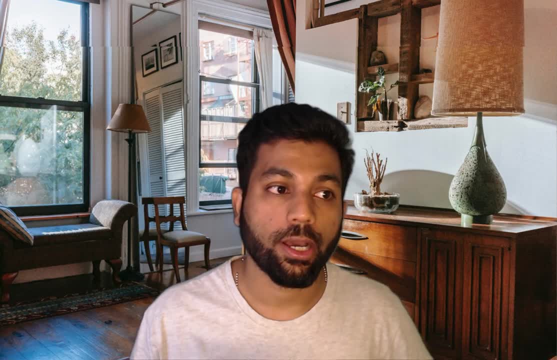 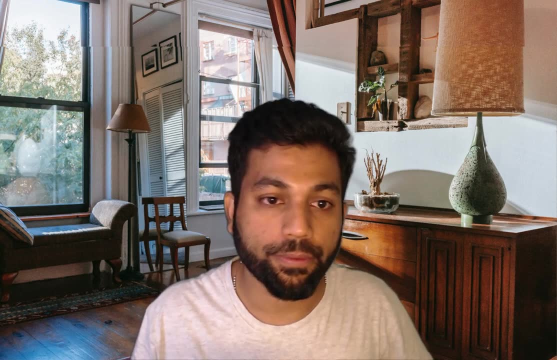 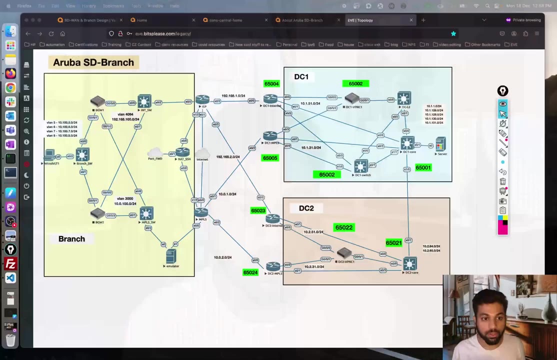 introduction video. so we will not be doing any major hands-on. We'll actually spend maybe the first 10 minutes just talking about the solution- right, a quick overview of sorts- and the next few minutes we will talk about the topology which I have set up. I think you can have a look over. 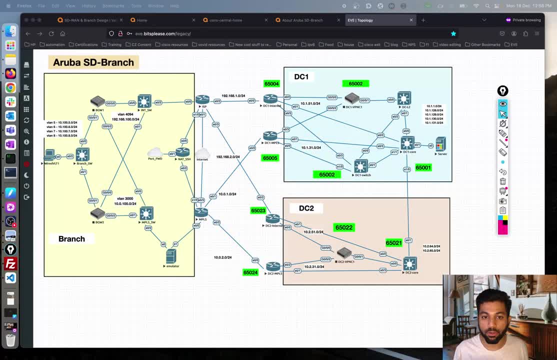 here, Right? so this is going to be the topology. So we'll talk a little bit about the topology and I'll also give you some tips on how to set this up. what are the prerequisites, and once we are done with that, we'll wind up, we'll come back in the next video and we'll actually start bringing. 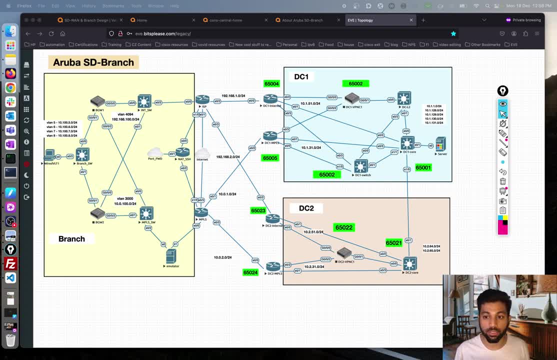 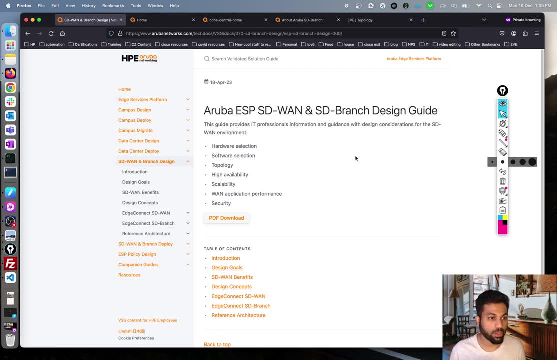 up these devices and bringing up the whole SDN solution from scratch. All right, okay, to start off, I think I've got a few links here. Let's open them up. So Aruba has this very cool validated solution guides And, as you see on the left hand side, they've got the guides for campus data center and the SDN. you. 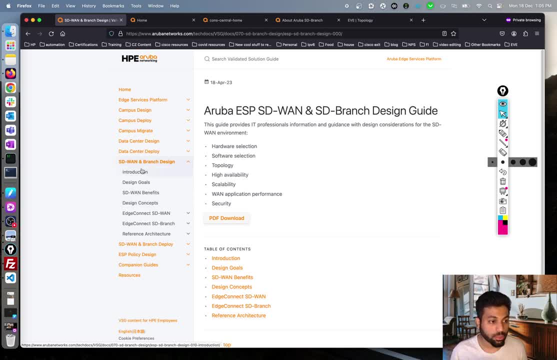 know technologies. So we will mainly be concentrating on the SD branch design section here over the next 10 minutes to kind of understand the solution a bit. We will obviously not be doing very in-depth analysis right now. We will do that while we do the labs. Okay, to start off, let's go to the section. 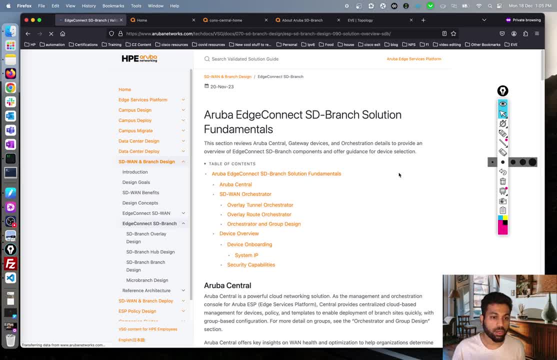 which is the EdgeConnect SD branch Over here, right, and let's try to just understand, right? So what do you kind of understand when you just see the word SD branch, right? So this was something very new to me as well, because I have worked on SDN right in data center, right in. we also have flavor of SDN in the land side, right. 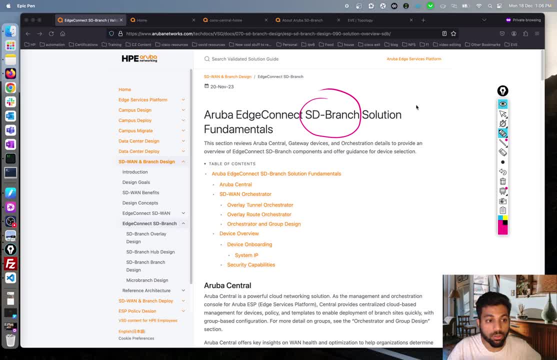 which was SD access solution in the Cisco's world. We also have talked about SD WAN right on the channel, Which was the Cisco's WIPTOLA solution, right, But SD branch was something, you know, something new, at least from a terminology perspective, right, But actually it's pretty simple. What does SD branch mean? It 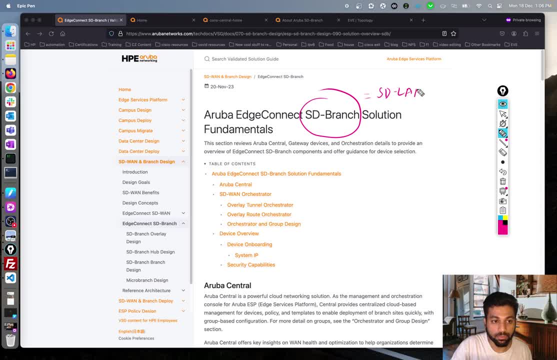 basically means it is SD LAN right plus your SD WAN right. It's just a combination of these two things which we and you have a convergence of sorts right, And that's that's where you know you're going to have a convergence of sorts right, And that's that's where you know you're going to have a convergence of sorts right, And that's that's where you 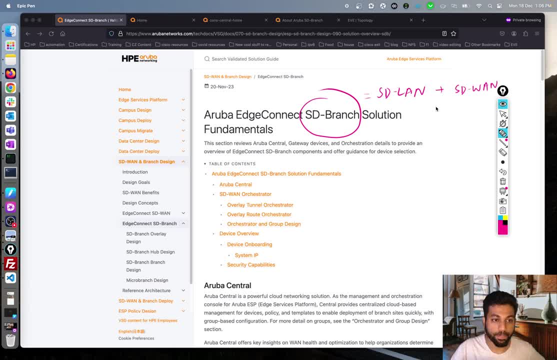 you know the term SD branch comes in. Now why do you have, why do you have a combination of this sorts right? let's try to dig that Now. when you think of a branch right, what what comes to your mind? it can be a sales office, it can be a small manufacturing unit, right it. 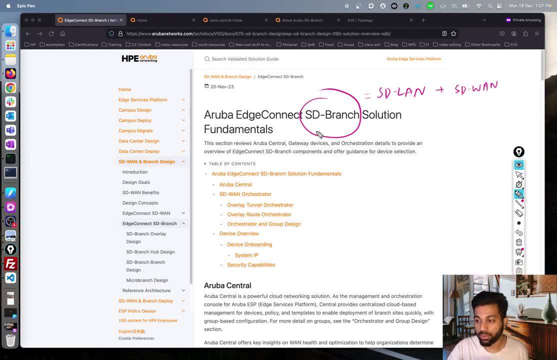 can be even store right, maybe a small, you know, retail store right, which can also constitute a branch. now again, when you imagine a branch, you've got, um, you know, a small LAN over there. right, you will need your typical wired connections, you need your typical wireless connectivity. right, you would probably also need a small ids ips a. 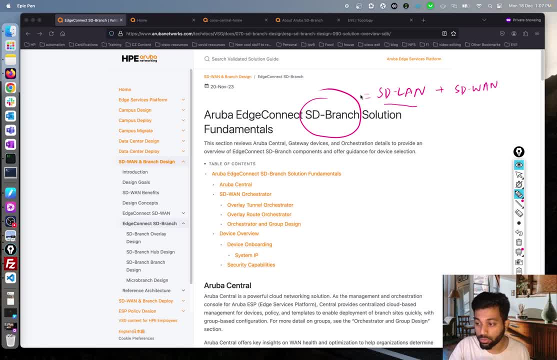 small firewall of sorts. if you have some, you know, filtering, which you want to do right, so that all constitutes the LAN. so how do you bring in the whole SDN flavor to that LAN? that's your SD LAN, right? SD-WAN? I think we again have spoken about SD-WAN in detail previously, but to just jog your: 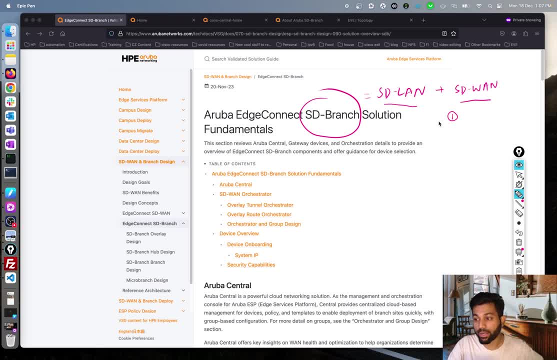 memory. what are some of the first, some of the two important things, right, two important use cases or problems it is trying to solve. one is trying to, you know, kind of get around the complexity of MPLS right. so MPLS circuits takes a lot of time to kind of bring up right. you also have cost. 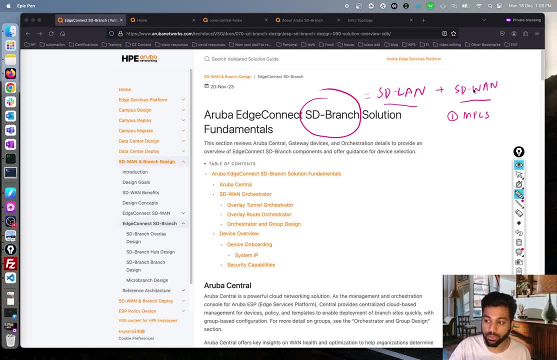 involved, right, a higher cost involved when it comes to MPLS circuit. so there are a lot of customers who are trying to offload the traffic from MPLS to a much cheaper options like the internet, right, and trying to use those transport. so you know, SD-WAN kind of enables you to do that. second thing is: 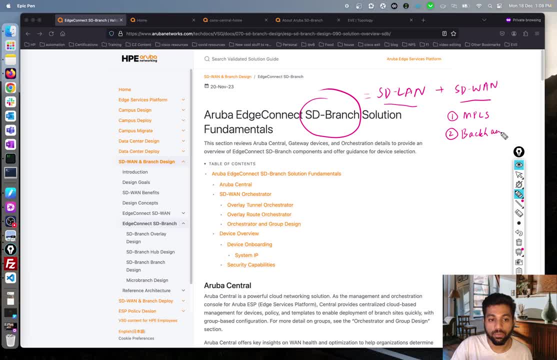 backhauling right. so when you see the word backhaul right, what? what does it bring to your mind? most of the applications. you know we are in 2023. right, most of the applications are moving to the cloud. right, and especially with the adoption of zero trust and so on, this has become quite you know. 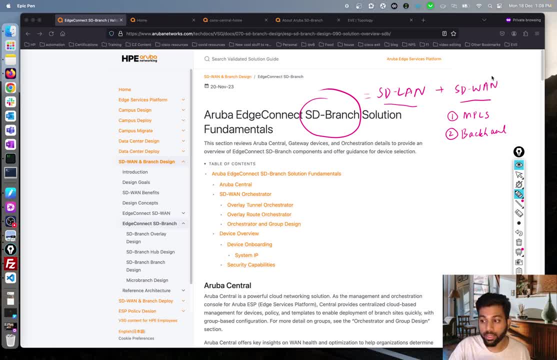 prevalent. so nowadays you know you will rarely see architectures where you know you have all the traffic from the branches being tunneled to a head end, which is like a data center. right, you'll rarely find that most of the applications because they are on the cloud. you know the network. 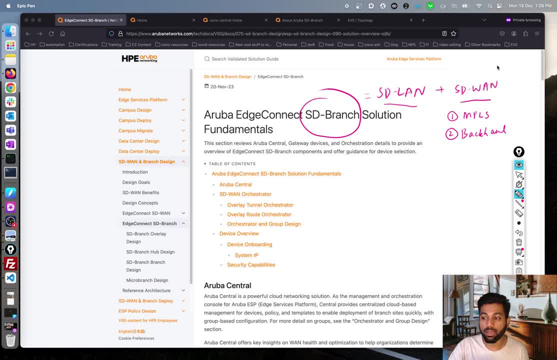 engineers prefer to kind of directly exit the traffic right, locally exit the traffic from the branches and go on to the cloud and do some kind of obvious, you know, edge filtering or do some kind of filtering on firewalling on the cloud as well. right, but predominantly people prefer to kind of 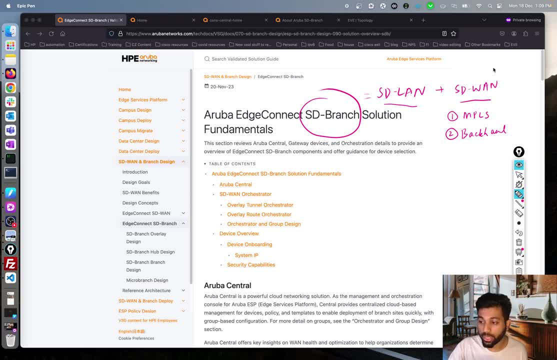 not backhaul the traffic all the way to the you know data center. rather, you know, send the traffic directly to the internet, since most of the applications are residing on the internet. now. these two are major you know pain points which SD-WAN kind of came into. you know solving it right. 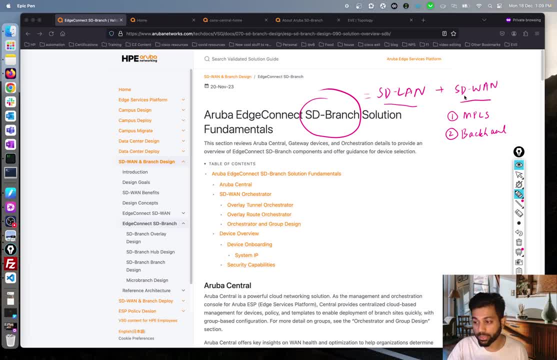 and that's that's kind of what it's been doing for the last two, three years. there are many vendors out there. you know you've got Cisco, you've got, you know, Aruba, you've got Fortinet and quite a lot of solutions which are providing the whole network right. so that's kind of what it's been doing for the 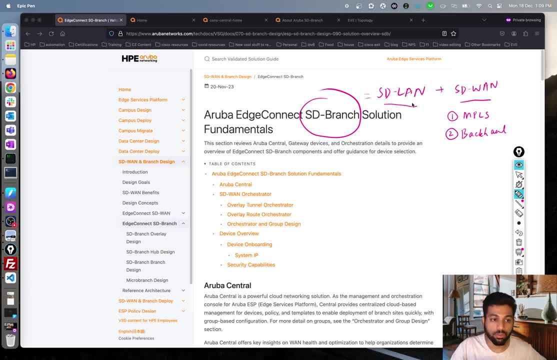 whole SD-WAN, you know, as a solution. so, coming back, you know, I think now we understand the whole reason behind SD branch. right, when you think of SD branch, think of it as having a solution which will help you to bring up a branch right, a small branch or medium branch, a larger branch, but at the 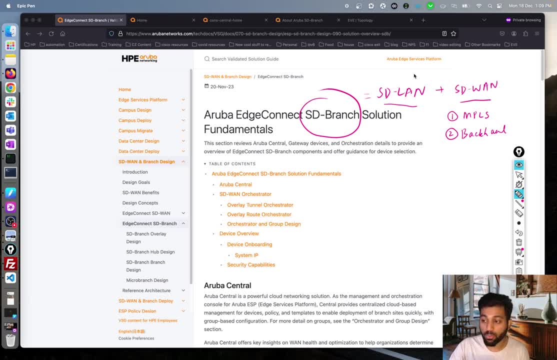 same time, you know something which is not just answering your WAN needs, but also the LAN needs. right, trying to answer, how do you, you know, bring up a branch, how do you bring up the wired connectivity, wireless connectivity, how do you do a little bit of filtering ids, ips? all of this with few clicks, in a software defined way. that is what SD branch is trying to. 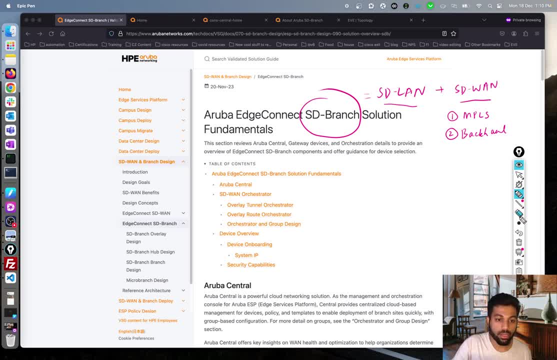 solve okay. so now that we got that cleared, let's try to see before before we. now, now that you understand SD branch also has a flavor of SD-WAN. let me bring up a very important point and kind of kind of answer your query, because on the left hand side you might see that there is a separate. 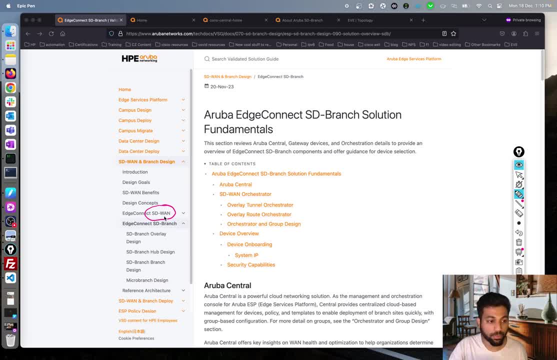 section called SD-WAN- right edge connect SD-WAN. so don't worry about that, because it's a separate section and don't confuse this SD-WAN with whatever we spoke just now. so this SD-WAN- what you see, the edge connect SD-WAN- is actually pertaining to another product, right, which is silver peak right. 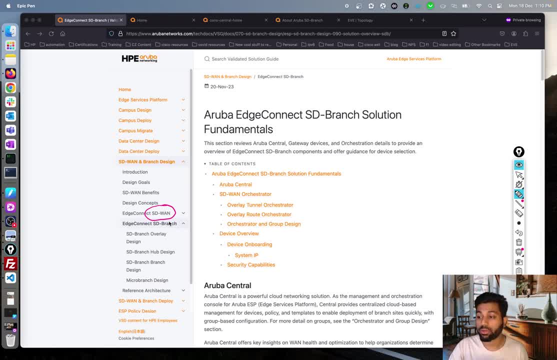 so Aruba also has another solution and product around the silver peak acquisition and the edge connect SD-WAN and kind of points to that. we will not be talking about this one in this video or in this series. we will probably do that in future, but right now we are mainly concentrating on SD branch. 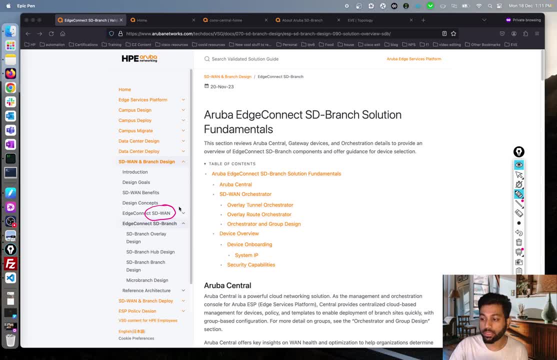 small flavor of SD-WAN to. it has some of the typical SD-WAN use cases, which we will be obviously covering, but these two are separate solutions. right, the SD branch and SD-WAN are separate solutions and we will be mainly concentrating on the SD branch. okay, so now. 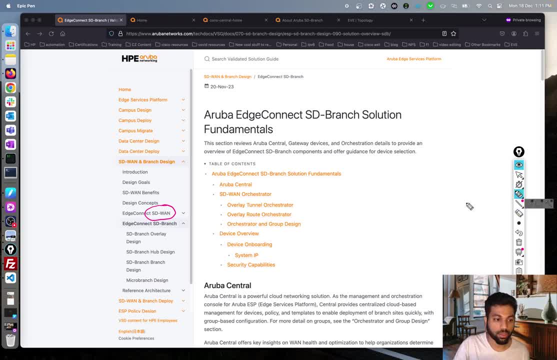 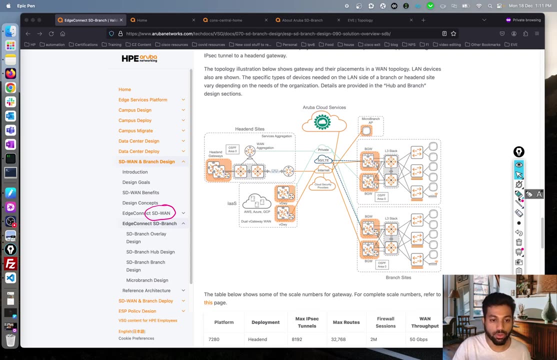 that you know that. let's actually come down to what. does you know what are, what are, various components of this solution, right? so let's see if I have a diagram here, yeah? so there you go. I think this is a pretty good diagram, right? so you know how to explain this. 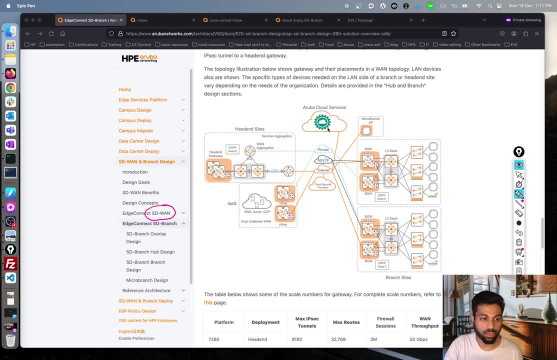 right, what are, what are some of the components? right, you see, here let's start from the underlay. whenever you talk about SD-WAN solution, you always have an underlay. you always also have an overlay right. so in the underlay you have typically what you've got your, you know circuits, right, you've. 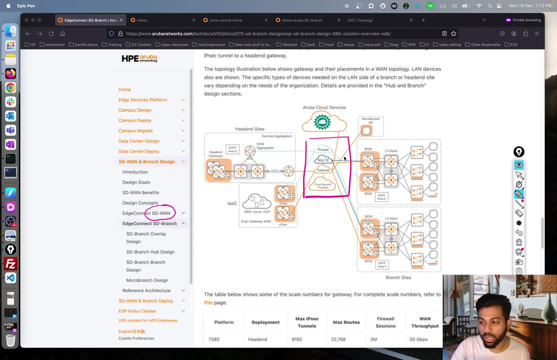 got your transports right, which is your. it can be your internet, it can be your LTE, it can be MPLS- right. so you have your transports, and then you also have your routers or the edge devices, right. so here you can see again, you have different flavors of edge devices in case of Aruba, right. in fact, there are. 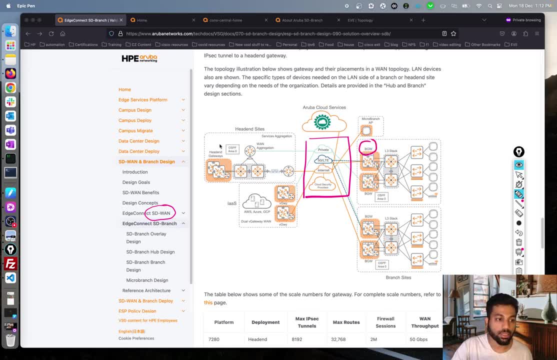 mainly two flavors, I would say. one is your branch gateways and the other one is your head and gateways. right, or head and gateways are also called as VPNCs, but predominantly these are the two flavors. right, so head and gateways are the two flavors. right so head and gateways are the two. 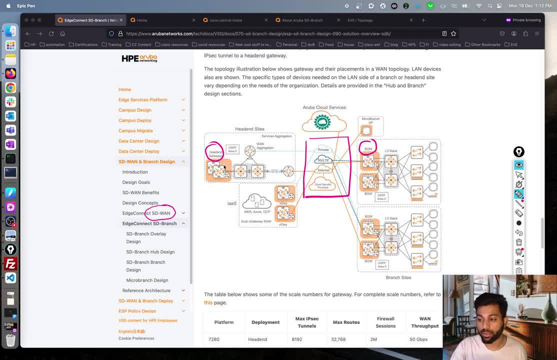 flavors right and gateways. think of it as those devices which generally reside on the hub side right, and they are. they are basically the devices where the VPN tunnels are going to terminate right, terminate from all the various branches, so they are like, think of it as an aggregated hub of sort. 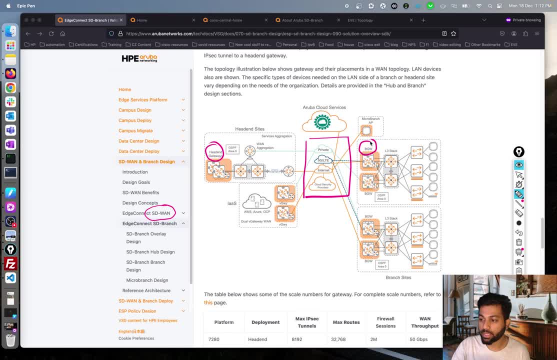 so that's your head and gateway, that's your VPNC. branch gateways are basically those edge devices which are going to reside in your branch offices or your stores or your, you know, maybe the sales, whatever you have right. so those are your branch, you know gateways from where generally your traffic is going to be generated, right, the users. 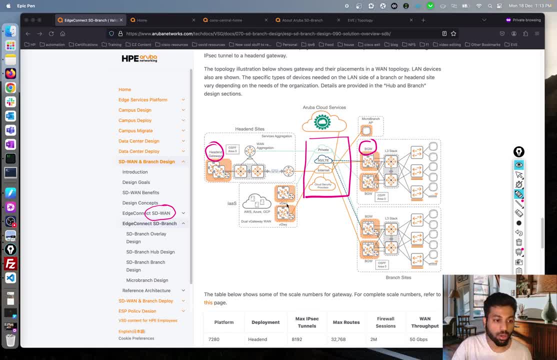 are going to sit in right. that's your branch gateway. you also have the virtual form factor. whatever we spoke now are physical form factors, but you also have virtual form factor, which your virtual gateway. now, these guys generally sit, maybe, in your ESXi. this is, they can also sit in your. 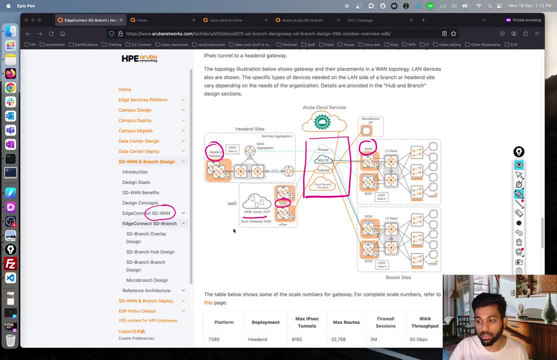 cloud, right, so which is AWS Azure GCP? they can generally sit there and that way, you know, you can have a multi-cloud strategy. right, you can? you can basically create a hub on the cloud and then connect all your branches onto the cloud and do all that fun. 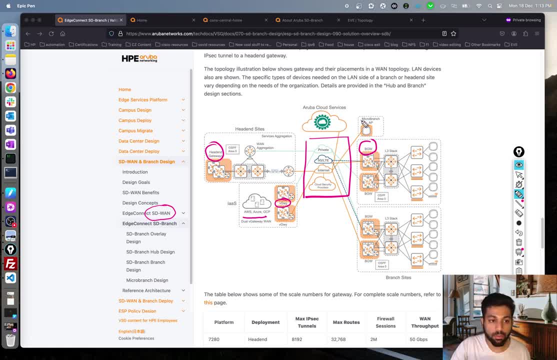 stuff. so that's another flavor. and the last one is you also have micro branch. this is again a very typical use case for an extremely small site of sorts right. so micro branch, think of it as an AP. but then you know, with few extra LAN ports of sorts right. so that way, you know, you can get. 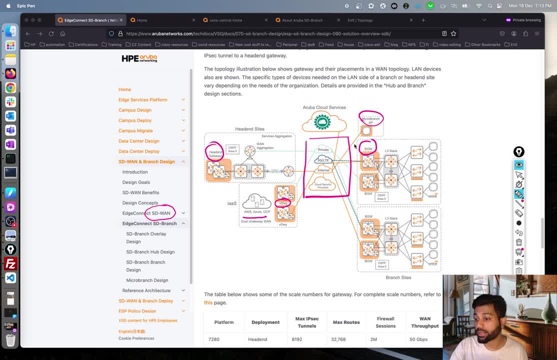 wireless and wired right from the single box, but at the same time it also has the SD-WAN capability. so you are getting the whole LAN and SD-WAN out of a small AP right. so that way, you know, you can kind of use this for smaller. 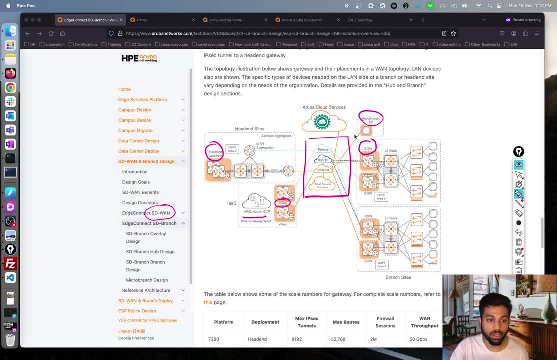 use cases like your home office and so on. right. so that's, that's another flavor. now there's one more important component, right. which kind of convert, which kind of puts all of this together, right, puts all of this into perspective, is your. you know what you see here on the center. this is: 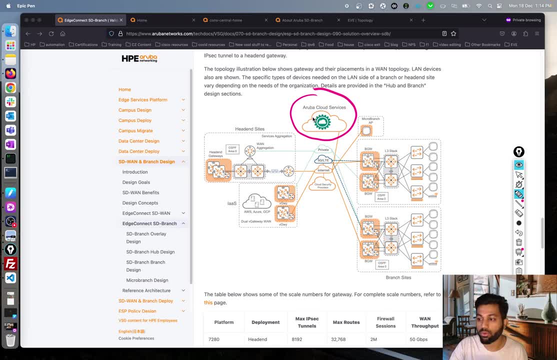 kind of like the main part of the whole solution, which is your Aruba cloud right, or or, in fact, in this particular scenario, I would basically call it as Aruba central right. so Aruba central is actually the think of it as a cloud-based, a SAS platform which does everything for you, which does: 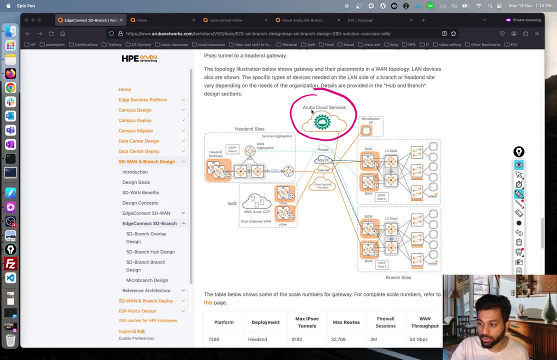 the management, which does the orchestration, does the assurance, monitoring of your whole solution, and so on. right, so, that's, that's why this whole solution, you know, fits in so beautifully for, you know, customers, especially those customers who who have a lot of experience with the cloud, right so? 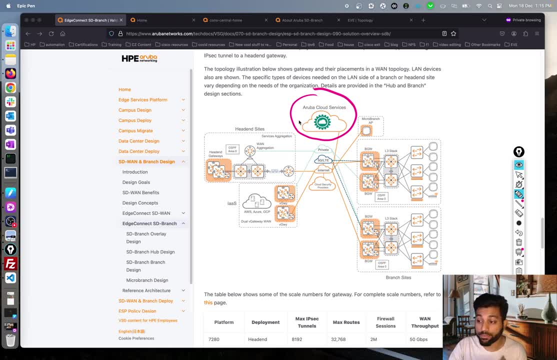 who have such kind of use cases, right like widely deployed a lot of number of branches across the country, across the continent, right, and they want a single pane of glass to do what to do? the LAN as well as the WAN right to manage, monitor, orchestrate their LAN, that is, you know, do some, some of the most. 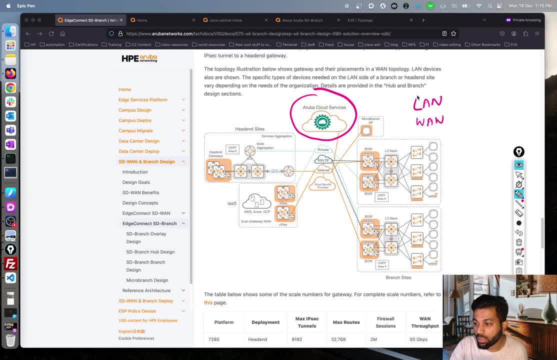 simplest things right. for example, create a SSID and, you know, advertise, broadcast that SSID at maybe 30 of your sites with a few clicks. you can do that. you know you want to kind of create a WAN policy or traffic steering policy right, and deploy it at maybe 50 of your sites with few. 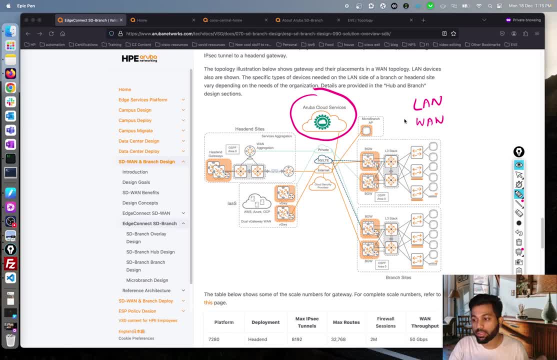 clicks you can do that, and all of this is possible because you have this centrally, you know, kind of administered, monitored, orchestrated solution, and it is sitting on the cloud right. so now, if you again, I always like to compare solutions, right, when I'm learning a new solution, I like to compare it. 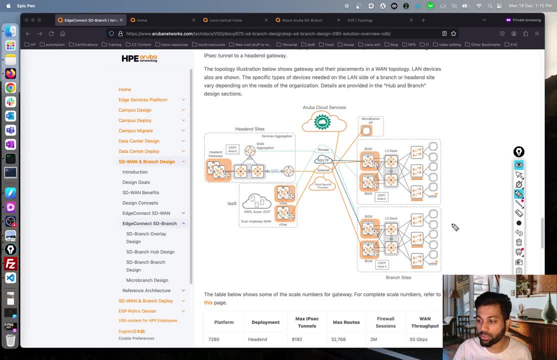 with the solutions which I've already learned. so if I try to compare this with my knowledge of other- you know- vendors out there, like, for example, Cisco's Wiptela solution which we have covered on the channel right, you will see, you will start seeing a little bit of similarities obviously. 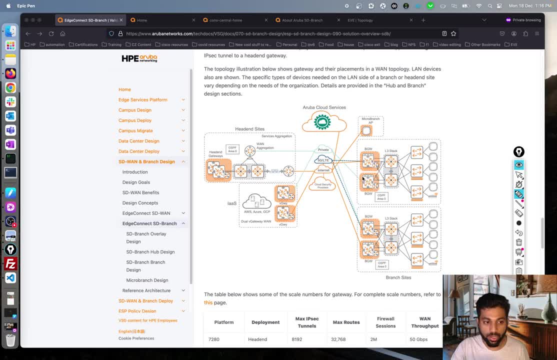 you've got the you know. from a devices perspective, I think you can already start seeing similarities. you've got the edge devices, you've got the transport. the main difference which I see here is in case of Cisco's Wiptela solution. we had a dedicated you know control plane, like we had a. 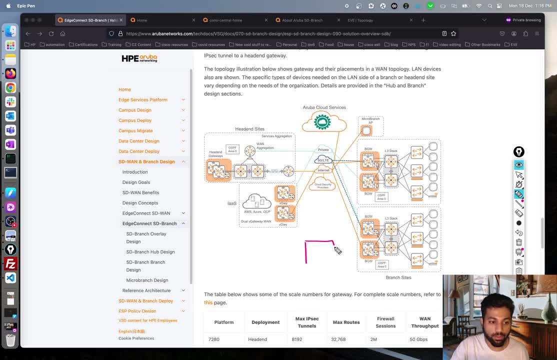 on-prem type of a control plane, right, we, we normally had what we call as Vsmart over here and all the edge devices they used. you know, overlay protocol, something called as OMP. right, you know, OMP was the protocol which was used and all the edge devices used to kind of. 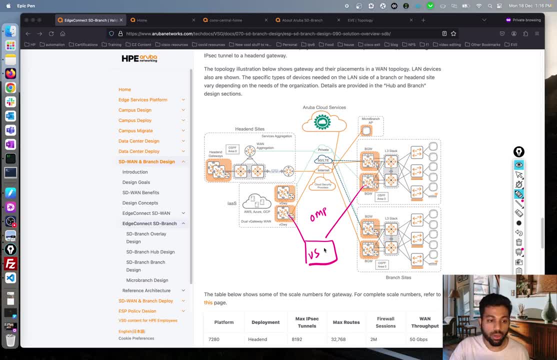 use this control plane protocol right to talk to the Vsmart right and the Vsmart was then orchestrating the tunnels between the devices. and you know, the OMP was obviously the protocol over which all the routes right for whatever the routes over here on the land side, right they were redistributed into the OMP and once you know the routes are, 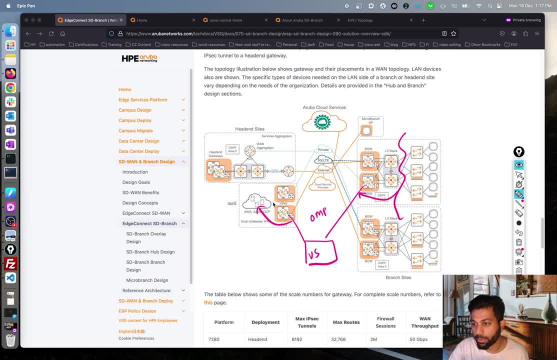 learned on the other side. they were redistributed back from OMP to, I don't know, maybe a OSPF, and so on, so that was the architecture which was there in case of your Cisco's. here also, there are similarities, right? so in this case, the main difference, though, is this control plane resides. 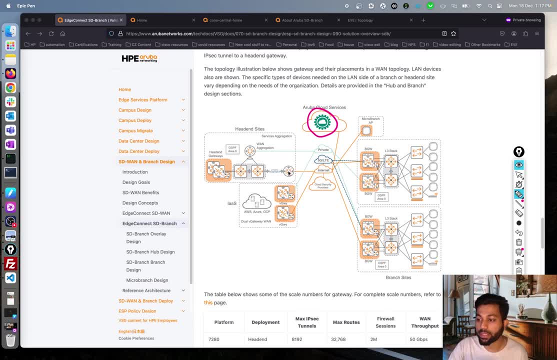 on the cloud right. you don't have to manage a separate appliance for it. you don't have a separate Vsmart of sort. the the control plane right is going to reside on the cloud, which means you know as soon as you go and you know orchestrated right the control plane is. 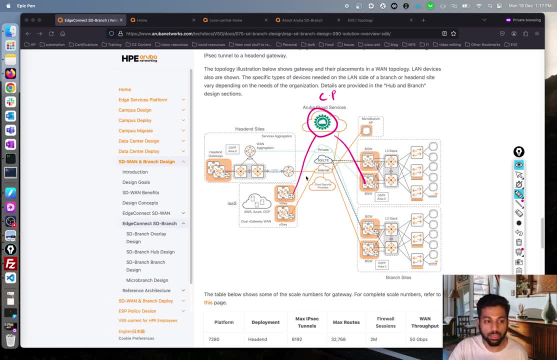 spun up. you still have like a overlay protocol, right, which is I think these guys call it OAP here- right, you still have a overlay protocol. so the rest of the architecture is still the same. I mean, you have all your LAN right subnets which are going to be redistributed into this overlay. 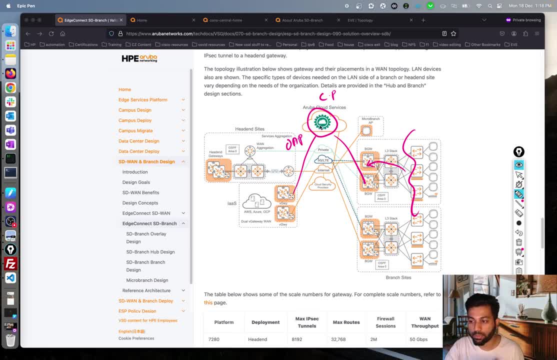 it goes all the way to the control plane. the control plane acts like a- you know BGP reflector of sorts, based on the policies, whatever you are configured, and the routes are basically learned right from the overlay protocol onto the other edge devices and from there they. 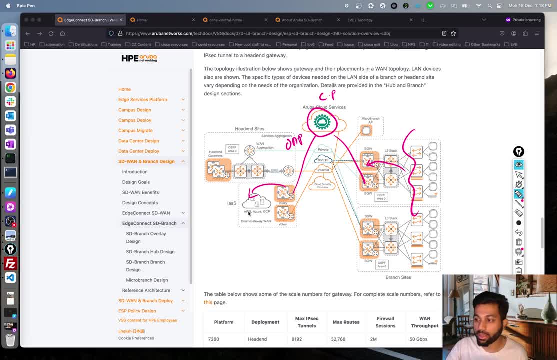 are redistributed into whatever protocol, whatever IGP are running, you know, behind the edge devices. right, that logic is still the same. the main difference is here. you will see, in the control plane perspective. the main difference here is everything is happening on the cloud. you don't have things like a vmanage, you don't have a vbond. you don't have a vsmart, a dedicated 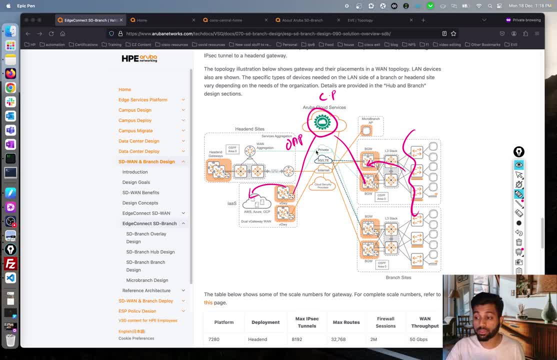 you know appliances which you would have the extra burden of managing, maintaining, upgrading here, everything this happening on the cloud. you know you, as a network engineer, you come in the morning, you open up your, you know console, your central, right, the central, the platform which is here, and you know this. 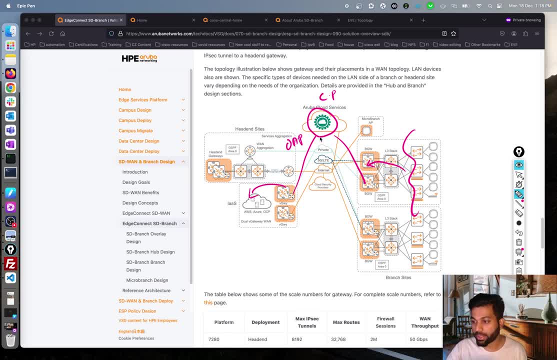 is going to be the place where you are going to do all your work. your day zero work. your day one work, day two work- all the implementation, deployment, managing, monitoring everything happens here. it also access the control plane right and Right, So all the devices will talk to it. get the routes, build the tunnels and so on. 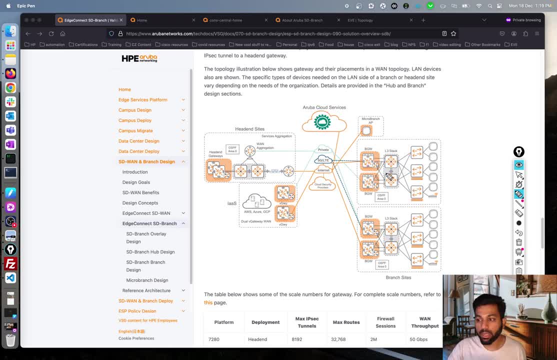 Right. So that's. that's the key unique thing from the data plane perspective, I think it's. there are a lot of similarities. Again, you still have the same IPsec tunnels Right. So between, so you know, you have different type of transports here: MPLS, Internet, LTE. 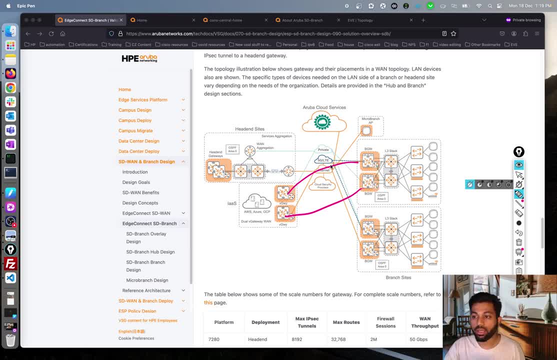 So all those transports, right? the edge devices will automatically create those IPsec tunnels, Right? So once you have those IPsec tunnels, then you know it's very easy to send the data traffic on top of on it, Right? So, yeah, So that's that. those are some of the similarities and differences between this solution and whatever we have already covered on the channel. 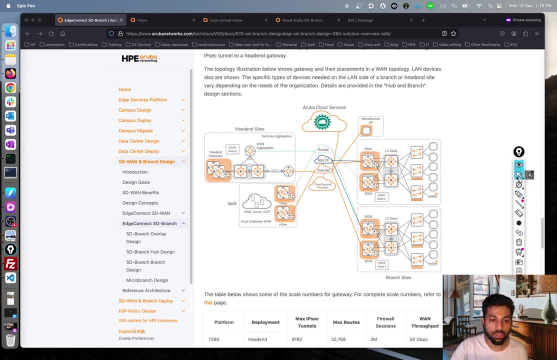 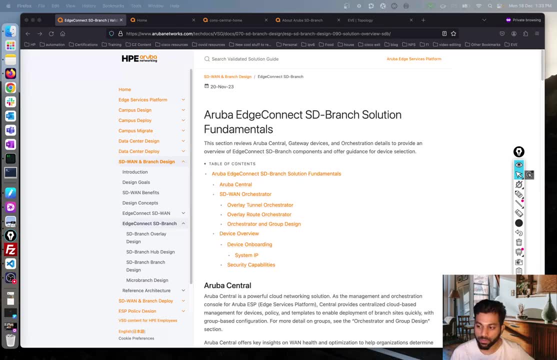 You have more details over here, So maybe we can quickly skim through those You can read about. this is again all publicly available information. I'll share the link so that you can read a bit about this. But All right, So we can now review the conference. 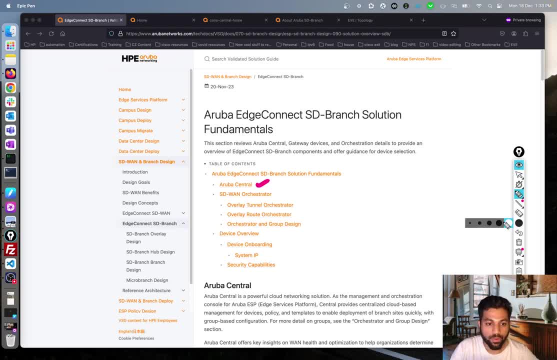 You can see that we have a number of different types of IPsec tunnels, right, So we have the central tunnel which we spoke of. As you see here, central is probably one of them. Right, Then, we already spoke of central orchestrator. 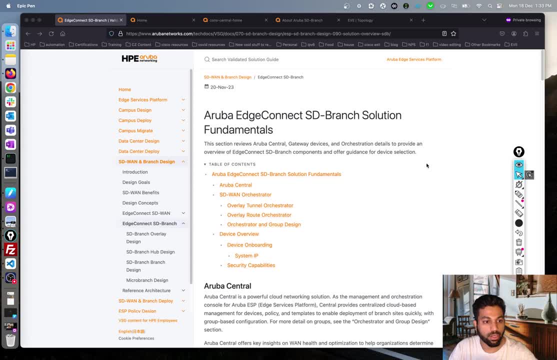 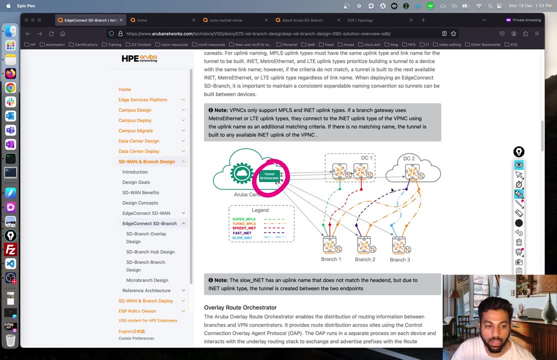 We already spoke of that. orchestrator is just a competent which is going to reside in the central. Maybe there is a better diagram here to kind of show that Right. So yeah, As you see here, this is the orchestrator: tunnel orchestrator. 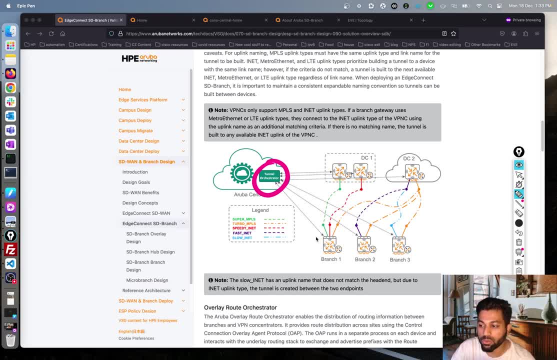 Right And, like we spoke, its main job is to create those IPsec tunnels, certain rules that you know: a tunnel which is created via the mpls connection here should terminate on the mpls on the other side, and so on. you know, you can read about those rules and 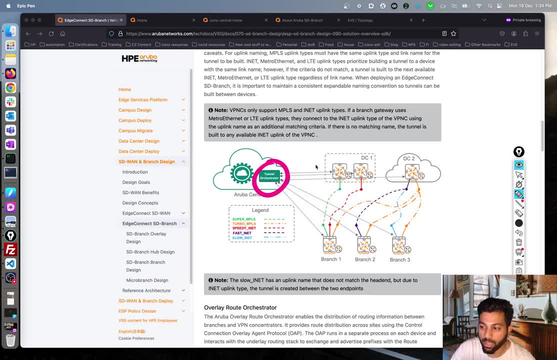 you know over here. but yeah, ultimately its main job is to create those ipsec tunnels, you know, those data tunnels on the overlay, which is where you know the traffic is going to finally get encrypted and be sent across the sites. right then, if you scroll down, you know if i will have the 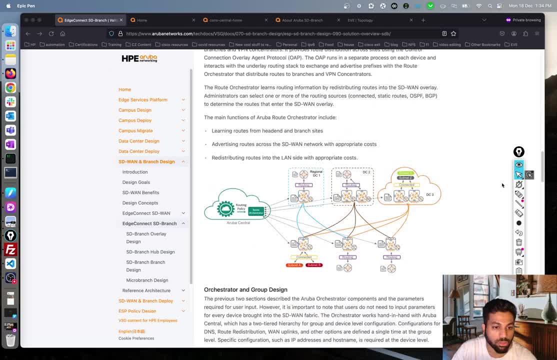 route orchestrator right. so, as you see here, the main job of this guy is again to make sure that the routes right, the subnets, in fact, right- uh, i use this pen- the subnets right, the, as you see, the connected subnets. or maybe you have dynamic routing, igp like ospf and so on. so all those- 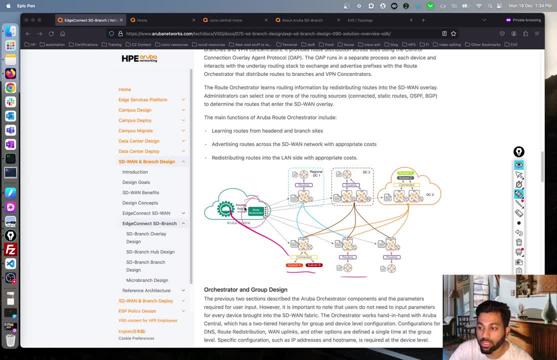 routes are sent all the way to the orchestrator, and the route orchestrator will act ո urgently in that way and you can get sent across the sites right. so that's why everything goes on the outside: access the environments when you're inside the floodplain, and all that's what is done. 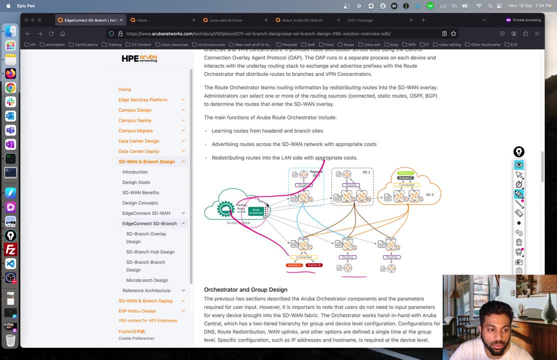 like a bgp route reflector of sort, and it will then, you know, send the routes to the, to the relevant sites, based on whatever control policies you have put here right, whatever route maps and so on, all the information whatever you have configured on the route orchestrator. you know it is going to. 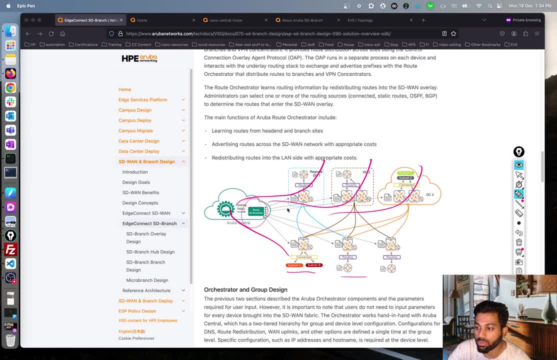 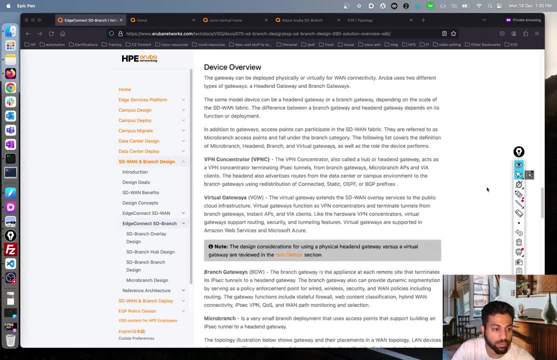 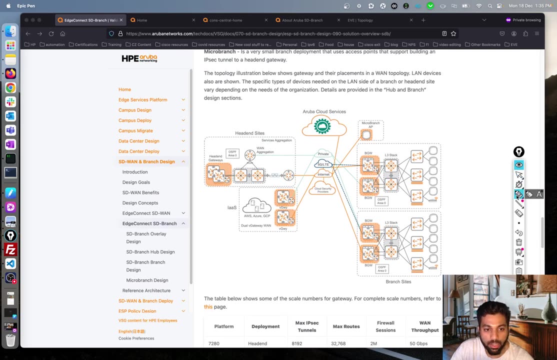 push the routes onto the remote sites based on those policies. right again, that's, that's mainly that. what else do we have here? we already talked about the components, the various components that make up this right. just let me spend a minute over here, right, because when you talk about the 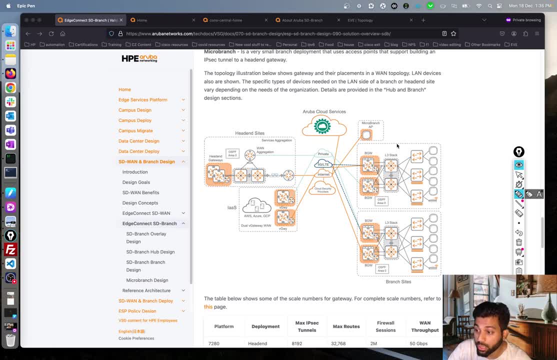 you know, when you talk about the aruba's ecosystem, if you're very new to it, right, it might take you a few. you know it might take you a little bit of time to get used to it. but when you look at aruba's ecosystem, they've got the- you know- obvious wireless. they are like a market leader in the 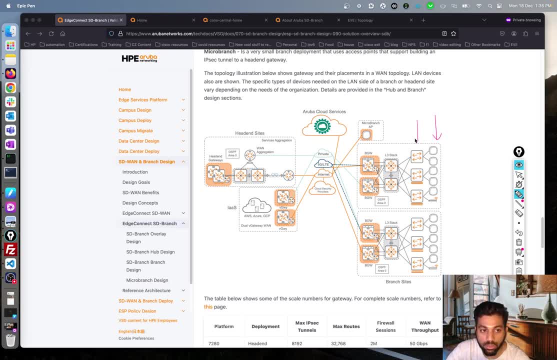 wireless space. they've got like very cool aps and so on. then they are also. they also have a lot of products on the, you know, access in the core layer. so that's, that's the first thing that we're going to talk about today, and then we're going to talk about the second thing that we're going to talk about today. 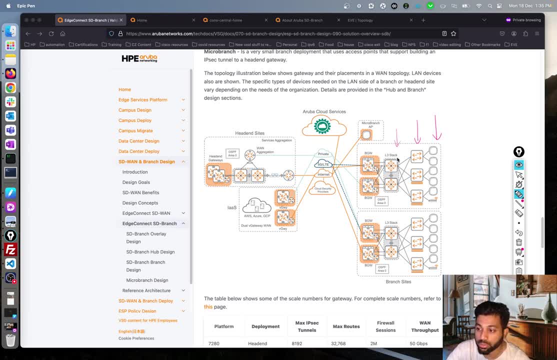 right, basically the switching right. they've got os switches. then they also have the newer os cx switches right. so again, if you're coming from the cisco's world, nothing new here, your typical access points, your typical, you know, layer 3 switches which you have. one important thing: 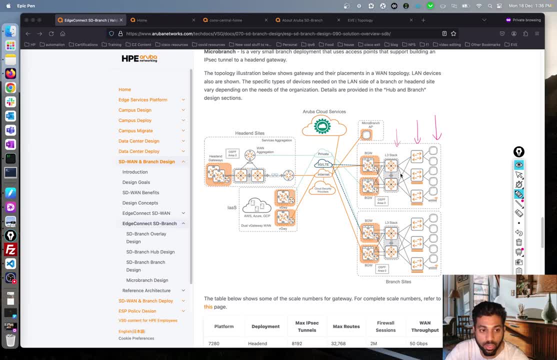 which, which i find again coming from the cisco's world. you know what i find? something unique here is you know the gateways right, so they have a lot of functionalities on these gateways. yes, we are right now talking about sd-WAN, so we are talking about the sd-WAN capabilities, but the gateways over here they are kind of like. 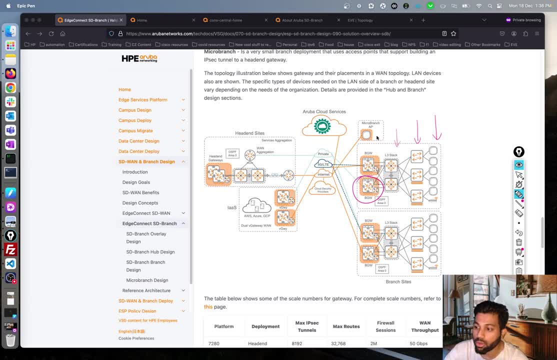 think of them as multi-talented entities. right, they can do a lot of things they can do. they can act as a wireless controller- right, they can do the wireless controlling controller capabilities right. they also can terminate wired tunnels- right, so the wired traffic which comes from. 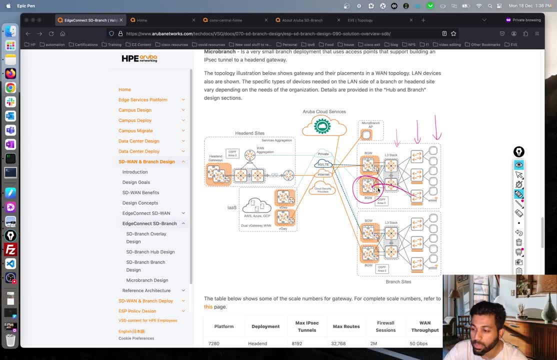 any of these access switches. you know you can create what they call as dynamic segmentation, so you can create tunnels all the way to this, gateways and you can do certain- you know- policy enforcements, you can do firewalling, you can do ids, ips, so you can do like a 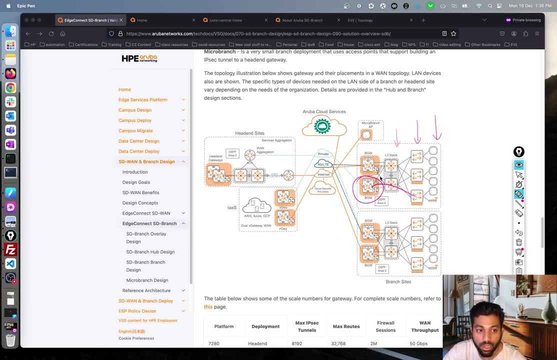 wired security policy enforcement as well. right, so they have a lot of, you know, multi. they're like multi-function gateways, right, you can do sd-WAN, you can do wireless controlling, wireless gateway of sort, you can do wired gateway and so on. right, we'll probably cover some of that in future. but 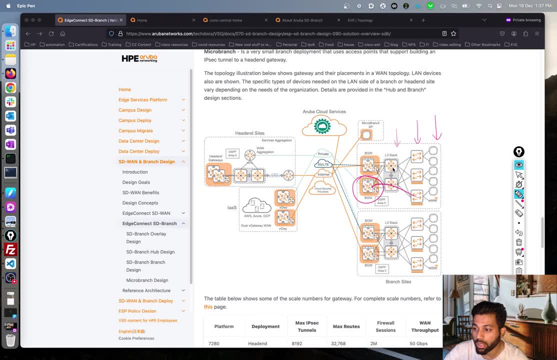 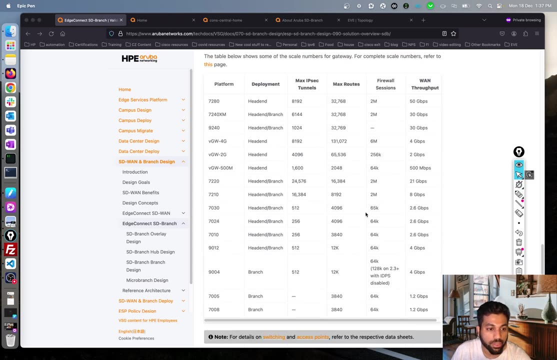 i just want to kind of give you a kind of like a quick glimpse that how this architecture, slightly how we did it. you know, in other vendors maybe like cisco right, cool. so that being said so, i think one last thing i want to call out here is we spoke about whatever we spoke. we spoke in a very general. 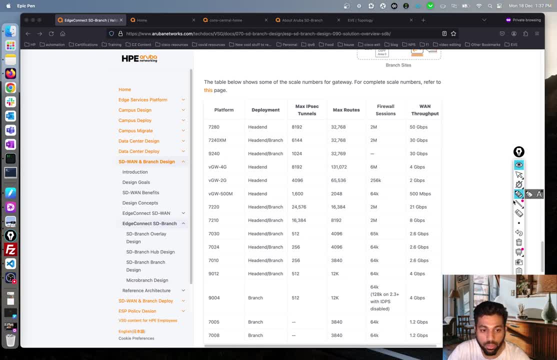 term. but when you look at the products right, you know what one thing you need to be very careful is. you need to be careful that the platform which you're going to use you need to check if it really supports that kind of a deployment, like, for example, here. the 7280s can be used only as. 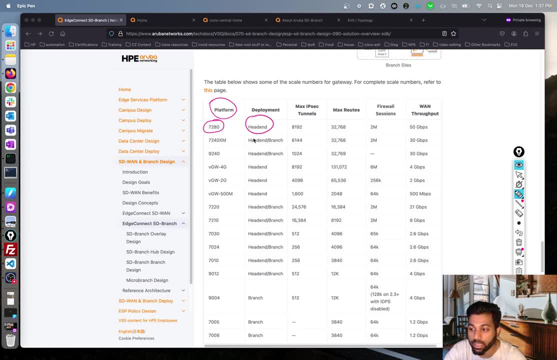 head-end device. we spoke about the head-end device. we spoke about the head-end device. we spoke about head-end and the branch gateways, right. so you need to be careful. there are some products which you can use as both head-end and branch, whereas like, for example, 9004, which is the product which 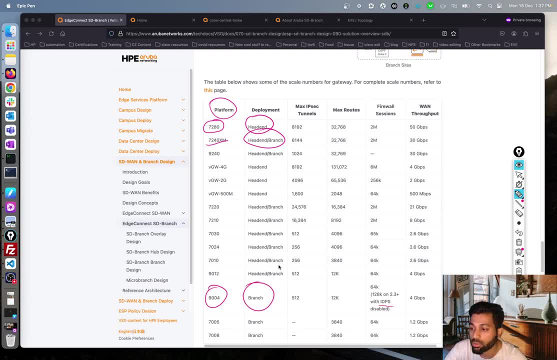 which supports ids and ips. right, that supports only as a branch gateway. you can't use it as a head-end. similarly, the pro. we are basically going to use virtual gateways in our labs, right in the evng labs. now, ideally, you should use them only as a head-end device, but we are going to use them as. 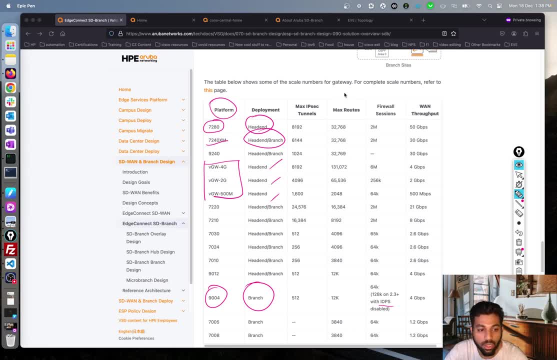 the branch gateway. also. it is not officially supported, but we are going to use it because that's the only way i can create a virtual lab right, but always make sure that you can use you use this sizing table to understand which device is supported in which deployment mode. 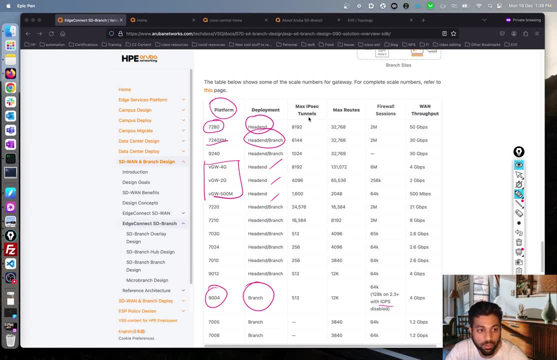 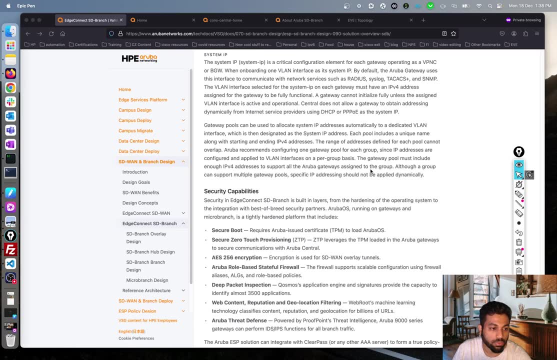 and what are some of the- you know, sizing charts over here, like, for example, maximum tunnels and so on. right, it's kind of important while you're designing this solution, all right. so one last probably thing is- maybe i think it's over here- which i want to cover is 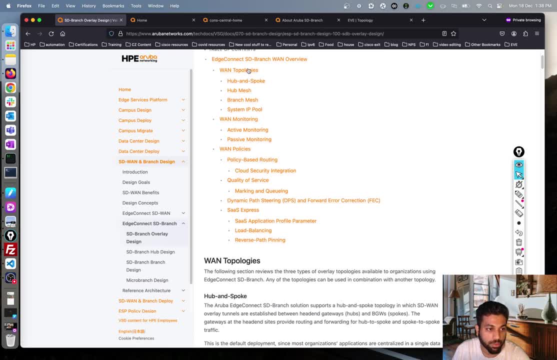 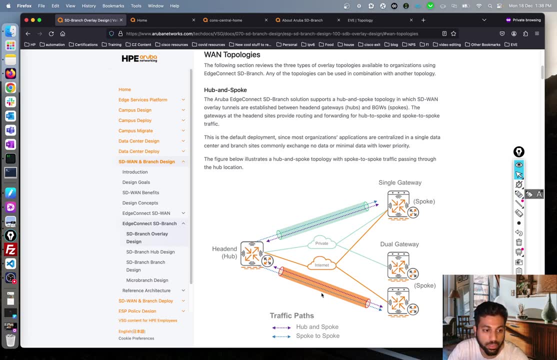 from a policies perspective. right, you've got again. maybe let me also show you the topology. so they also have different type of topologies which you can create right. the most common one obviously is the hub and spoke which you see here right. where the spokes can't talk to each other, all the traffic from the spokes goes to like a hub. it can be a regional hub. 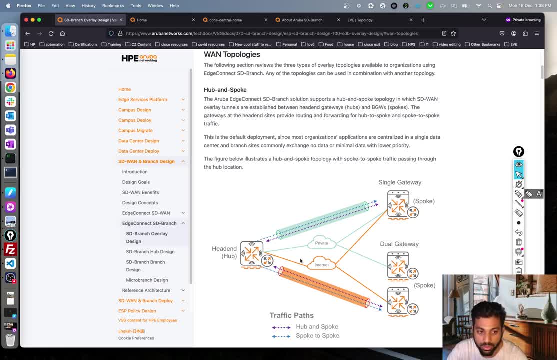 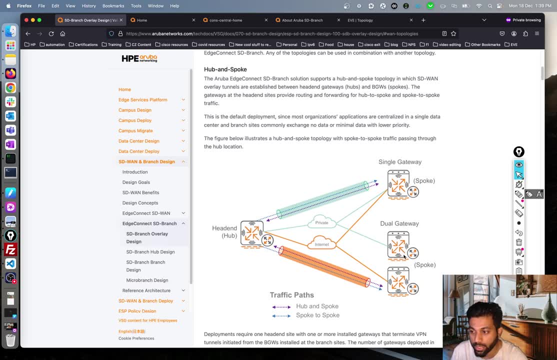 or it can be like a universal hub, but yeah, so this is like one of the most common uh topology. you can also do, obviously. you can do all types of redundancy. you can put multiple gateways at the branch, you can put a multiple gateways at the head end and all of that. 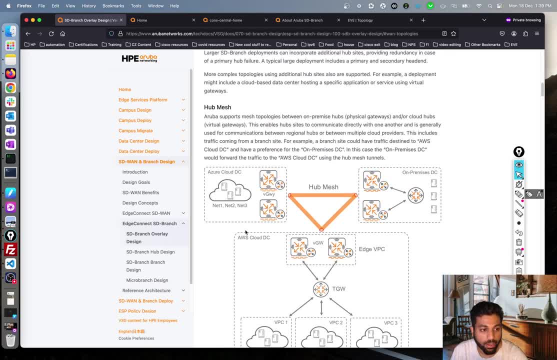 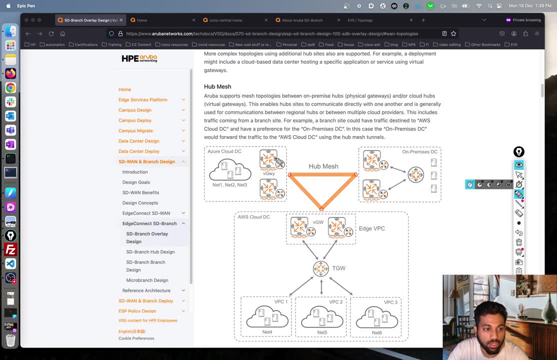 we will talk about some of those deployments while we do the lab. but in addition to that you also have some other deployments, like a hip, like a hub, mesh, right. so you can see, here this could be a typical deployment if you are a very big enterprise, right, you might. 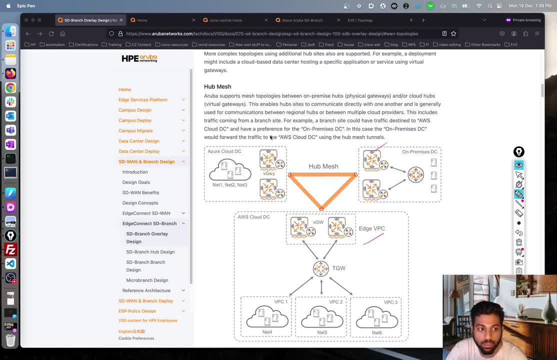 have a hub in singapore, another hub in sydney, other one in london and you want like a full mesh, full routed mesh between them so that you can send a lot of traffic between this, maybe like a disaster recovery right. you might have like three data centers where the hubs are located and you 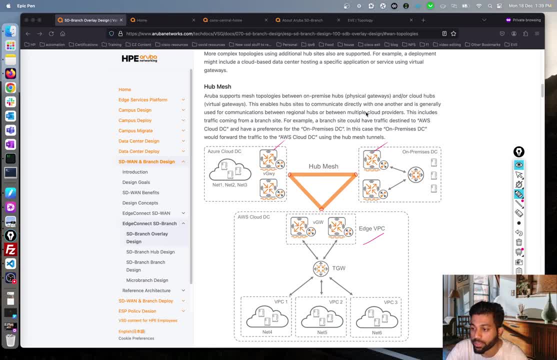 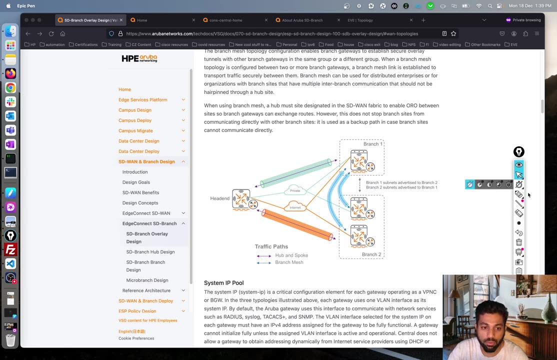 want like a disaster recovery between them. uh, you want to send a lot of terabytes of data between them. then you want a full- uh, you know- mesh of sort right, so you can create a, you can create that kind of a topology. then you also have your branch mesh right. so if you, if you have a use, 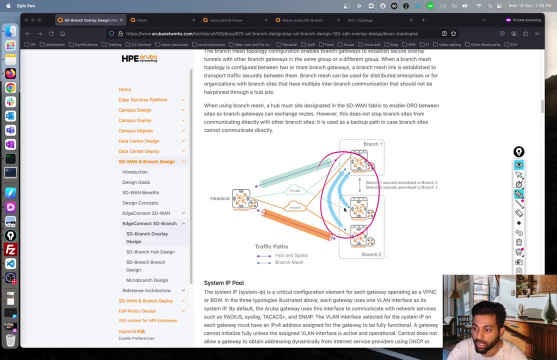 case where you want, where you really want your branches to talk to each other, right, um, and kind of deviate from your typical hub and spoke, you can do that as well, right, using uh branch mesh, so you have such kind of multiple topologies based on your use cases, um, and one last thing which we are 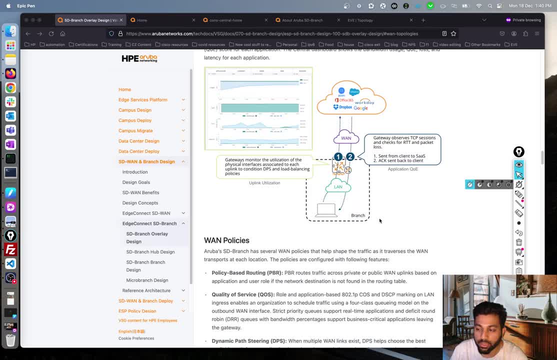 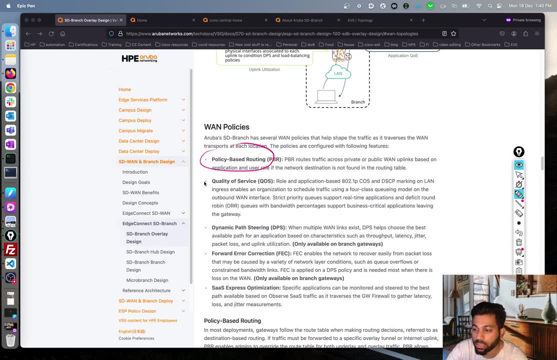 which i want to cover here is uh policies right, just like any other sdn solution. here also you can create very extensive policies like shown here. right, you've got your typical policy based routing pbr right for doing things like direct internet exit, local breakouts and things like that, where 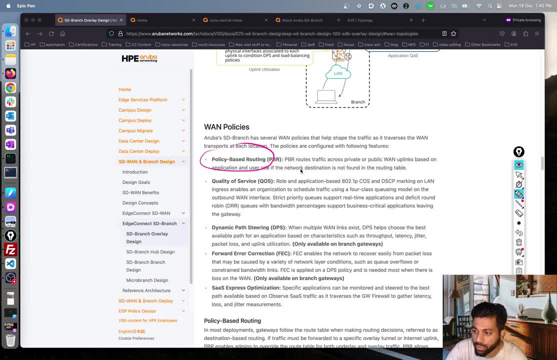 you match the traffic based on certain classifiers, right, and then, once you match the traffic, you can then decide what is going to be your next hop right. so that's what you can do with pbr. qs is very much important again, because we are talking about van here. 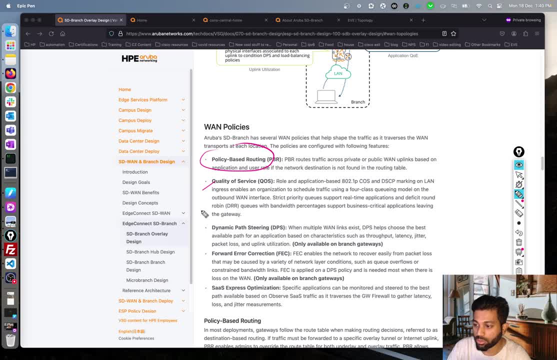 right. so you really need shaping and polishing to be done at your edges. so i mean, you normally do shaping at your edge as the enterprise agent, then the service provider generally does some kind of policing. but yeah, if you have to do shaping then you might want to also do some kind of marking and 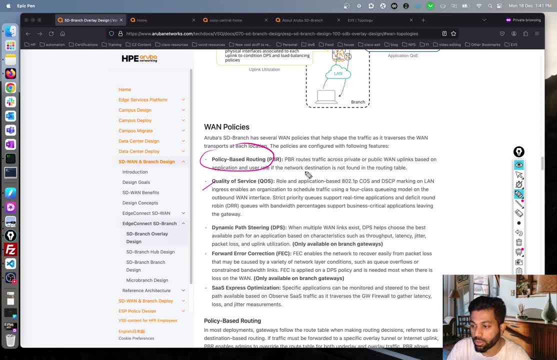 all of the, all the normal classification marking and all of that which we normally do in qs, right? so all of that can be done here: dynamic path steering. so this is again, if i want to take a resemblance here, right, the dynamic path steering is actually actually very similar to application aware routing, which we 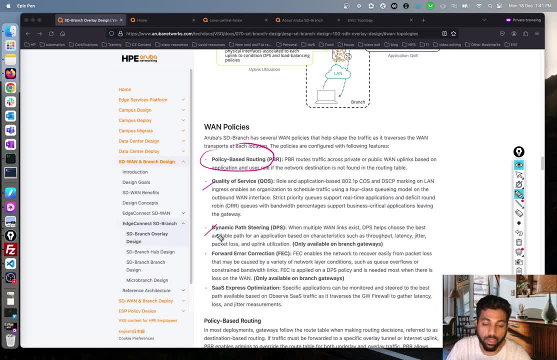 kind of did in, you know, in cisco's hd van whipdela right. so this is again something where you can kind of create slas right based on throughput latency, jitter, packet loss, and then you can let the device, the branch device, decide what uplink it is going to use. you know, 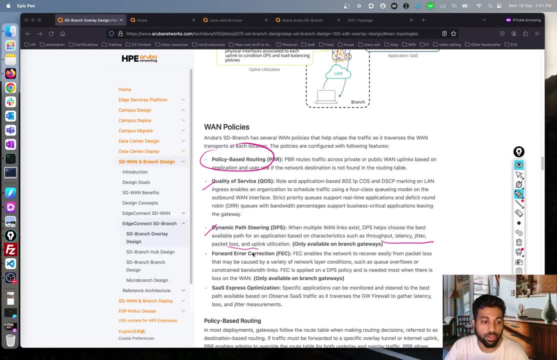 which is going to meet these slas right. so it's very similar to application aware routing right and then forward error correction, again creating you know when you're sending the traffic. you can insert some parity packets. that way, you know, you can reduce the number of free transmissions and all of that very much of a vamin optimization technology and you. 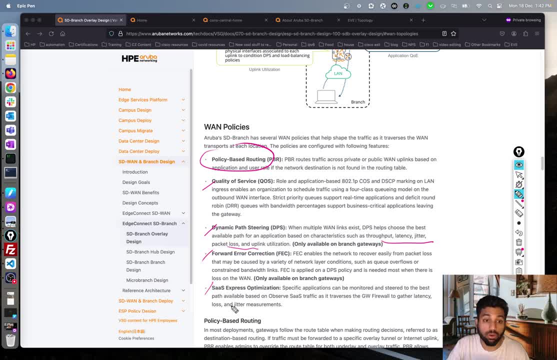 also have sas express optimization. this is very, very similar to cloud on ramps right. so, especially the sas cloud on ram, which we already did in whipdela right, where you can send, you know certain probes right to some of the. you can send you know certain probes right to some of the. you know certain probes right to some of the. 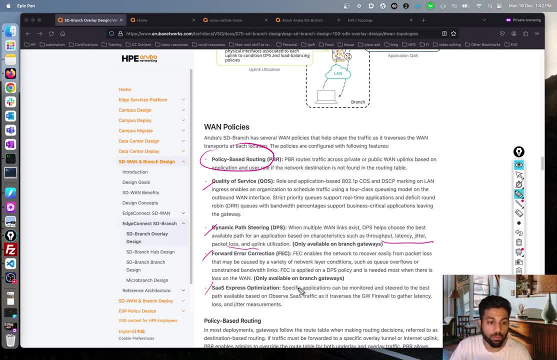 popular sas applications, right like dns probes, http probes, and then you can let your edge device decide which you know path it is going to use to talk to that particular cloud provider. so yeah, those are various policies which you can kind of set up in your sd branch solution. perfect, so. 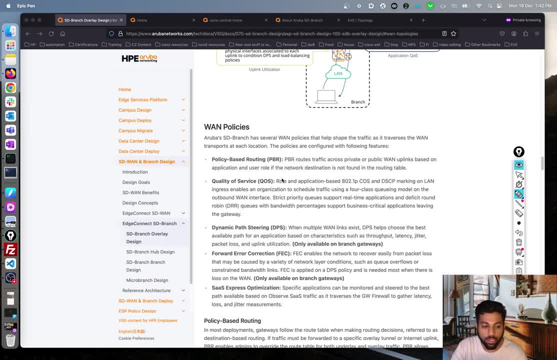 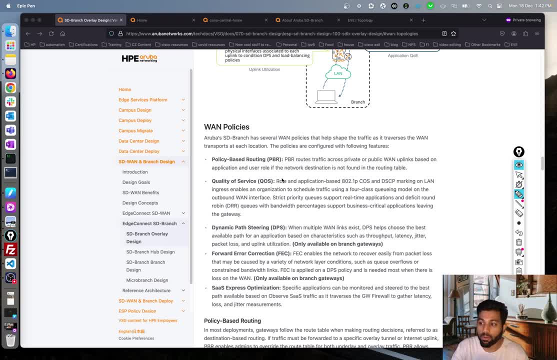 how the overlay is created, right, and we also talked about the policies part. we also talked about a little bit about the various types of topologies which you can create here and the policies- right, the different types of policies, because that is the ultimate goal of sdn, right. 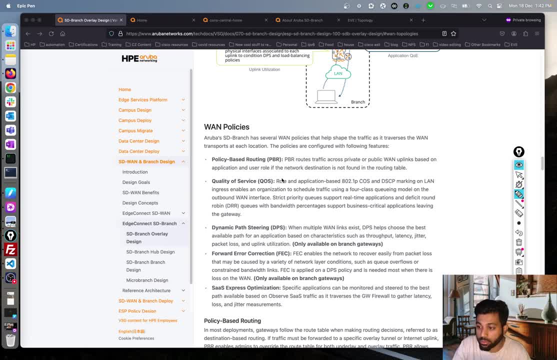 you should be able to kind of steer your traffic with few clicks right, you should be able to steer your traffic over mpls or internet based on certain matching criteria. that is what you can do ultimately with most of the sd1 vendors, and that's what you can do here as well. perfect, moving on so. 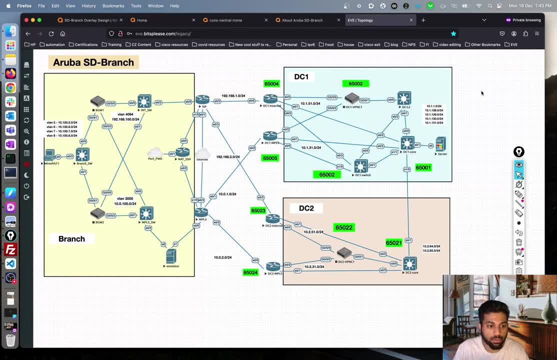 let's move on to my topology over here. so it's going to be the topology, right? just to give you a quick understanding of everything here. so, you, this is going to be one of our branch and we have two data centers here. right, our branch gateways are here. we have two branch gateways. these are: 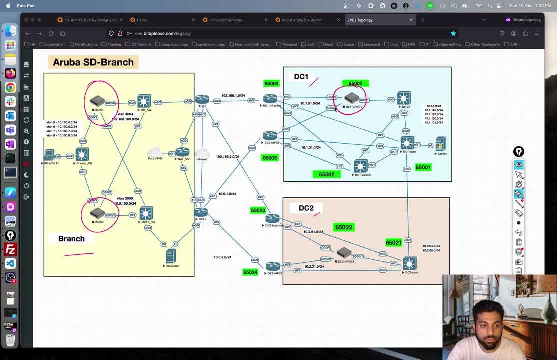 the aruba's virtual gateways and you also have the same virtual gateway here as the vpnc's right. ideally, we should use the virtual gateway only as vpnc and not as branch gateway. we are using it. it is not officially supported. we are using it because it is just a lab. rest of the stuff is. 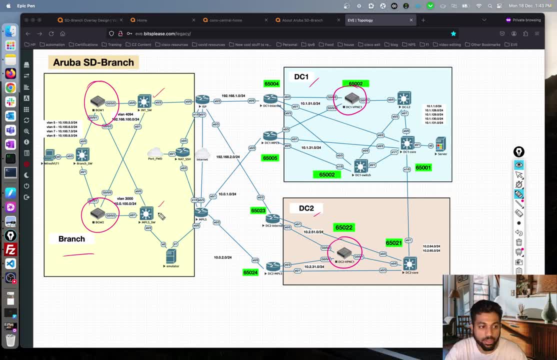 again. you see you have like a l2 switch here, right internet switch, mpls switch, um, you know where you know, which is basically where you have the multiple which is ultimately connected to the internet isp provider here. similarly, you have the mpls provider here. what i'm trying to do here is 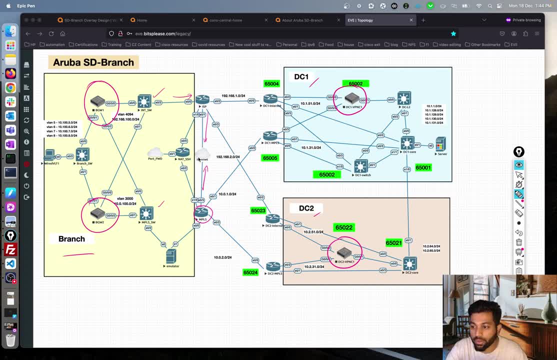 um, send all the internet traffic right. i'm using even g's capabilities here to kind of um use um. i'm basically natting all the traffic out to the internet, right so that, so that my vm over here has connectivity to the internet. uh, nothing very complicated this, like you. 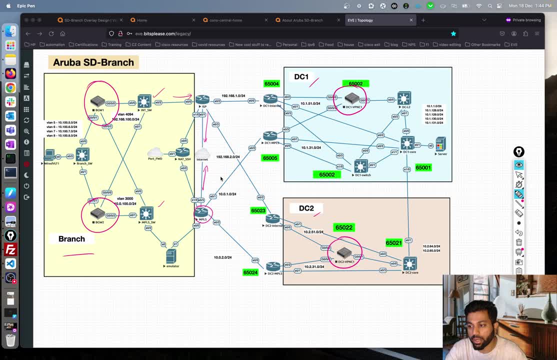 have a lot of tutorials on how to do this and i think even g documentation also kind of is pretty useful to do this um you also have. i also have like edge devices, like isp devices, mpls devices at each of the branch- sorry, each of the vpnc um on in this particular dc one you will see a lot of. 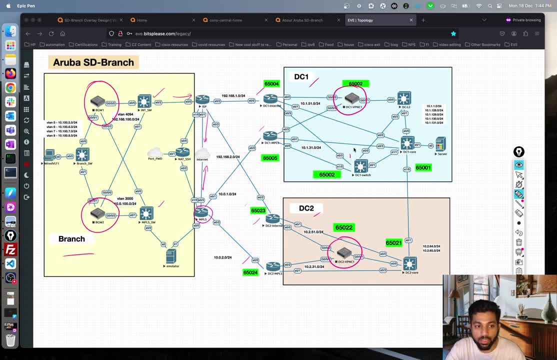 extra devices, because i wanted to add more devices here to clay, to kind of show you bgp, and so on. so you can see there is a dc1 switch, there is a dc code switch and so on. this is just an l2 switch because i i have just one port here, so i wanted to put a l2 switch and, uh, you know use. 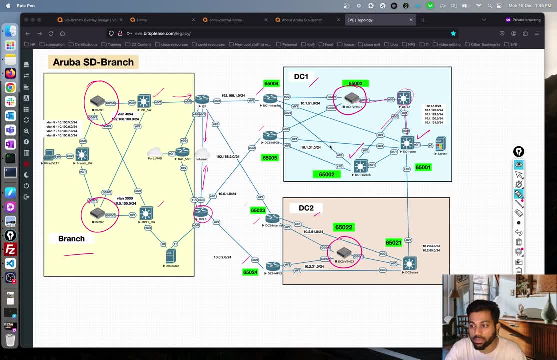 vlans to kind of create two bgp neighbors, right? that's why i've added this l2 switch, similarly on the dc2 side. again, it's a small side, so i have just one dc core switch and these are the subnets, right, you can see various subnets at all the three sites. ultimately, what we'll be doing is we'll be. 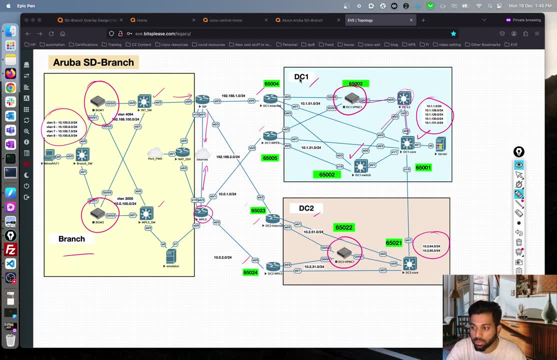 able to talk between these two sub, these subnets. right, that is the whole goal. bring this whole thing up and then make sure that all of these guys are able to talk to each other. then you know, obviously we will do some. you know, policy-based routing. we will try to influence which uplinks. 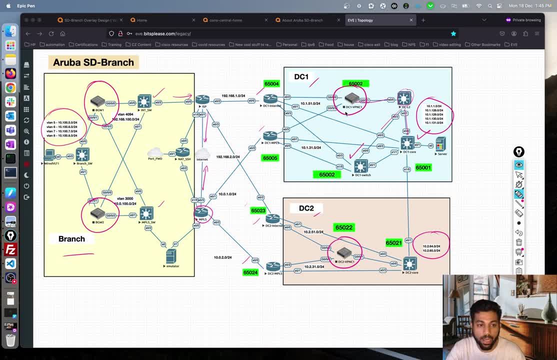 the traffic is going to take and all of that, all the fun stuff. that's what we'll be doing in the lab series, but i just wanted to give you an introduction of what, how this topology works. okay, now the next important thing is so we will not mainly talk about the rest of the devices here. 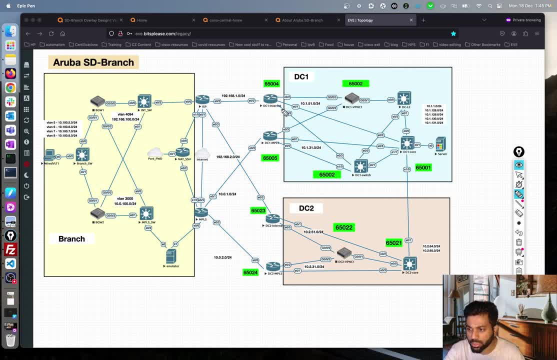 like, for example, the switches and routers. those are i'm using. i believe i'm using virtual ios or iol routers here. right, very straightforward stuff. we will not be talking about those things. i will provide the configurations of those devices on my github repo once the whole series is done, so that 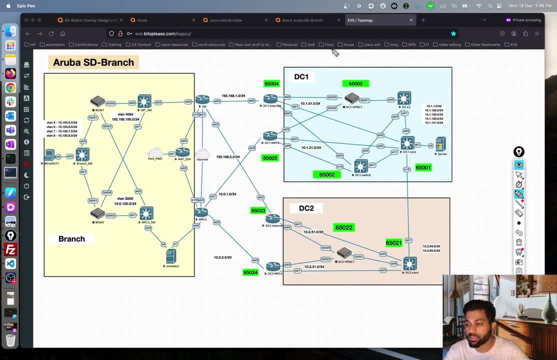 you can like, use my even g file. you can use the configurations and start with the lab immediately. you don't have to figure out all the addressing and stuff i will. i will give you all of that. we will just concentrate about how to bring up a virtual gateway, right? so? 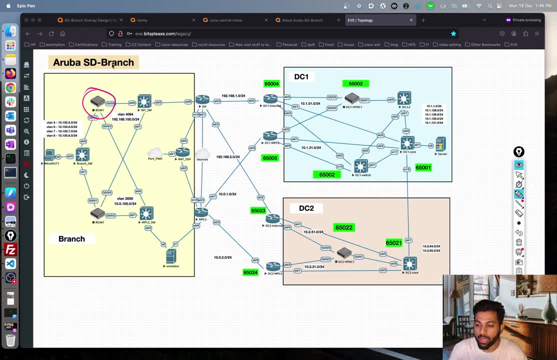 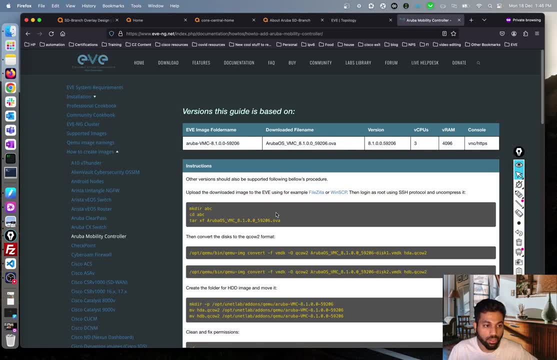 what you need for this, right? so let me just grab the link for that, okay? so if you actually go down to this, if you go down to this, even g's documentation- right, there is a section for aruba's mobility controller. so i'm basically for. i followed the same procedure. 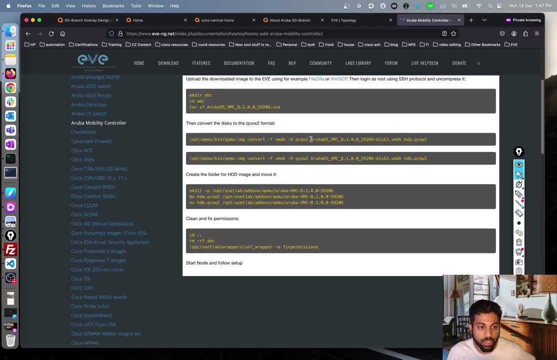 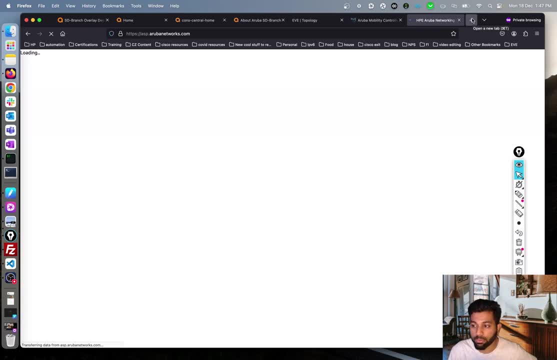 to kind of get the virtual gateways up right. all you need is, um, you need to go to asparubanetworkscom. this is. this is where you can download all the software which you need, basically the virtual gateway. i'm using the 8.7 version, uh, for for the labs you can use 8.5, 8.6 or even the 10.x versions. 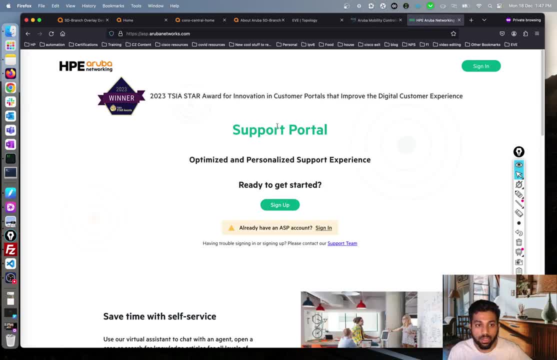 uh, you know most of the stuff should be same right. so this is where you will need to download the software from. i will not be able to provide the software because that would be kind of illegal. so if you don't have access to download the software, maybe reach out to your aruba partners or aruba. 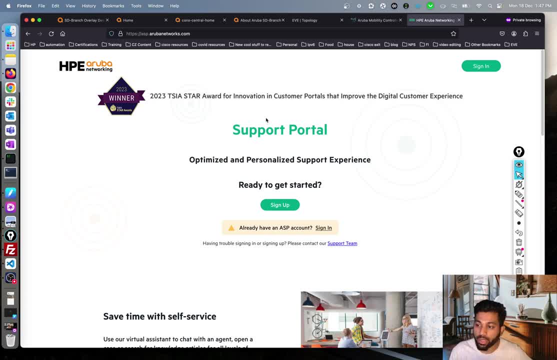 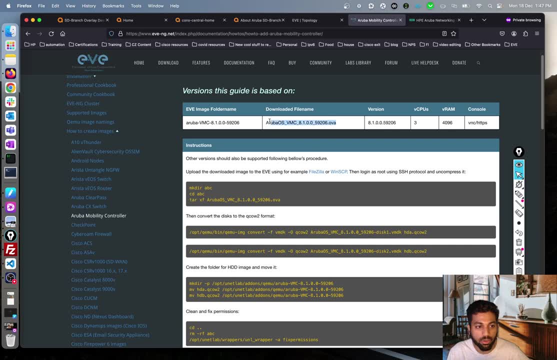 account managers and they should be able to help you kind of get the software and get you started to explore this technology. um, that being said, yeah, the process is pretty straightforward. you will be able to download a file which is very similar to this ova file. right and um, the ova. 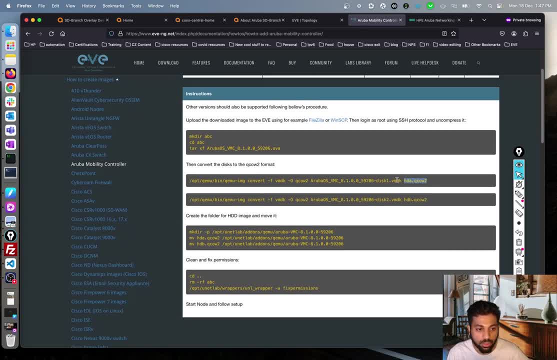 file can then be, you know, converted into. like you see here, you'll basically, when you double click and open the ova file, you'll get like two disk one is your disk one and disk two, and then you just need to use the same process here mentioned to create the 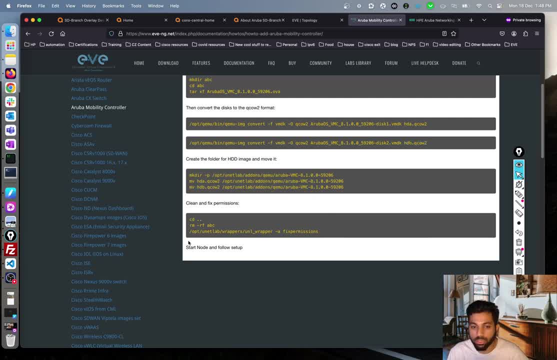 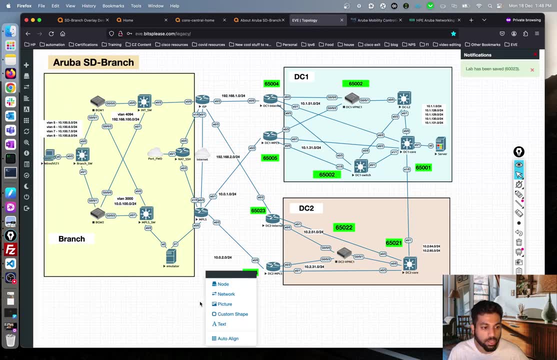 two hdas, um, and you know, follow the naming convention and then move it right. so once you do that, the device will show up. uh, one interesting thing is- i don't know if i can let me show you- so- one important learning for me over here was: once you go and add a node like, for example, the device, 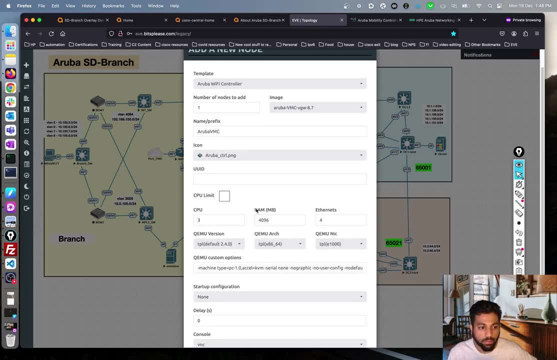 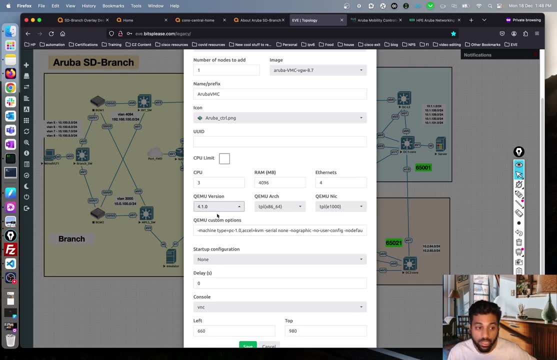 right, and, as you see, i'm i'm using 8.7, but one important thing is: make sure that you change the keymo version to 4.1, right? because, um, if you don't do that, then you know you will find your devices sometimes getting stuck and so on. so i've had that issue, but once i moved it to 4.1, you know things. 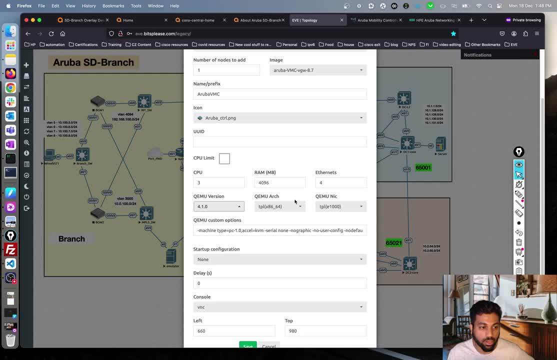 were pretty simple, right? the next important thing is: yeah, you can use the ram ethernet and whatever i've used here. always make sure you use just four ethernets over here, because the more number of interfaces you add, i saw that the device is not going to be able to do that, so i'm going to use 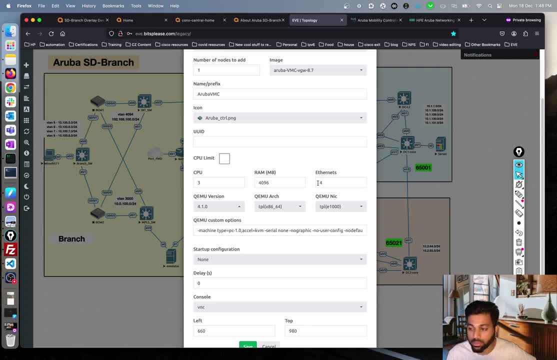 just four ethernets over here because the device was not booting up, so i made sure that the interfaces were fixed to four. um, you know, and if you want to create more interfaces, you can use concepts of vlan to kind of, you know, trunk, trunk the ports and virtually add more lan ports, right, 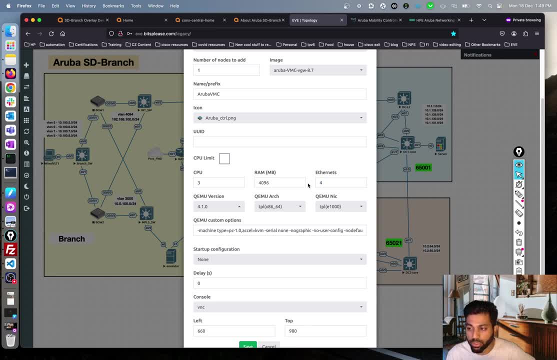 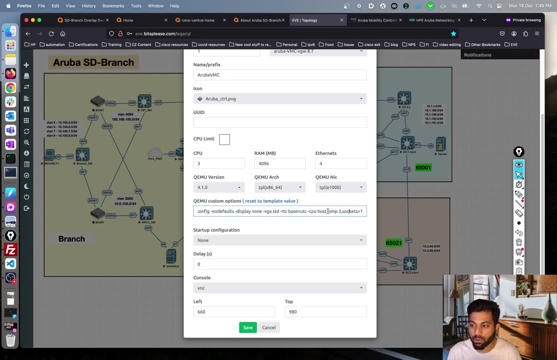 so you can use that logic, but make sure they use the ports port number to be four. the next is the keymo options. right? so at this moment, what i'll do is let me just pause my video and let me just show you what exactly keymo options i use to make this work. okay, so i've pulled up the keymo options, right, so i'll 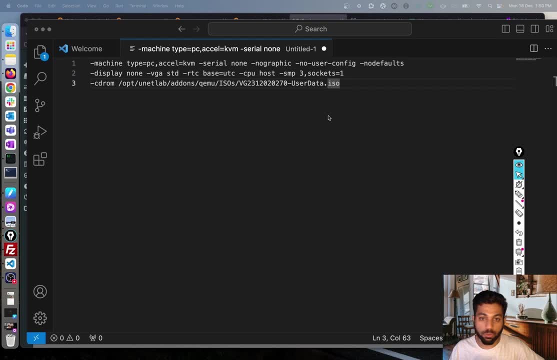 obviously paste this in the description as well, but just want to kind of this act this: all the three things should be in the same line, right? i've just broken it down to multiple lines just to show it to you, but the whole idea is that make sure you copy the exact keymo options, right, and 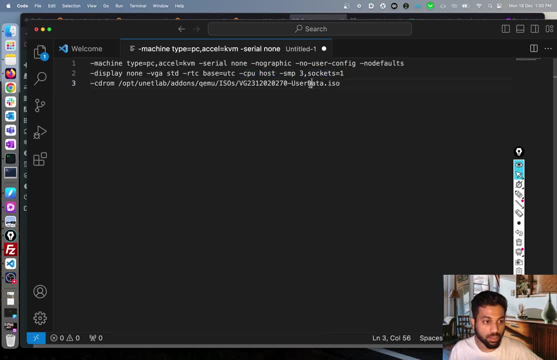 you might ask me a question: what is this cd-rom right? because you know, you see there is some kind of iocpc right, and i'm going to copy this cd-rom right, and i'm going to copy this cd-rom right. so this is a keymo option, so you can copy that one from an iso file over here. and this is this is. 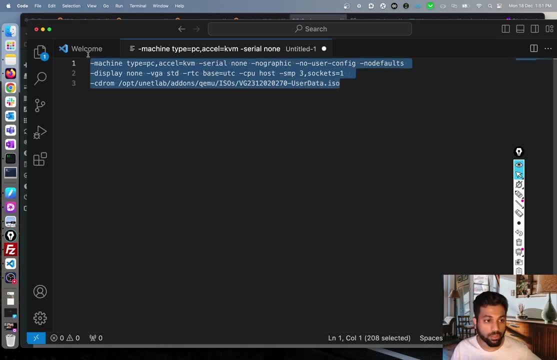 one other important thing for you: to set up the lab right, so you need this metadata file right, and i'll tell you how to get it. but for a minute right, just try to look at this one. make sure you use the exact same keymo options, otherwise things might not really work. all you have to do is you know. 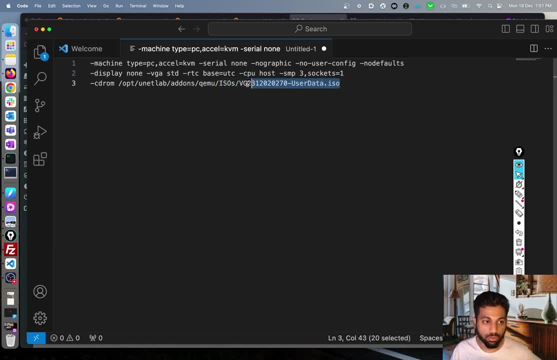 copy the whole thing and then replace- you know this- this section which is the isos and the iso folder and the iso file. basically, you will need to generate these metadata files from the iso file if you can use them, for example, for some other purposes. if you need to generate some other things, you can also do it. 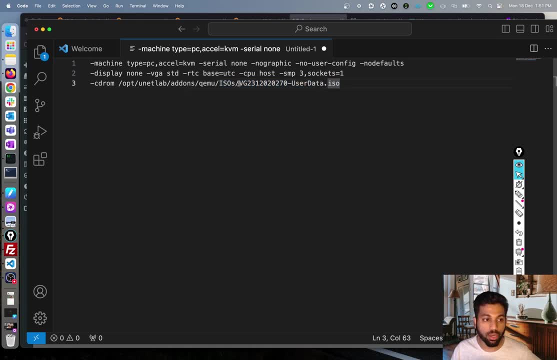 you know aruba central and you need to upload these isos to your- you know even g, and then you just need to use the dash cd-rom flag to point it to those iso files. that's it right, and i'll show you now how to generate those. um, you know iso files, right, so let me take a minute here, okay. 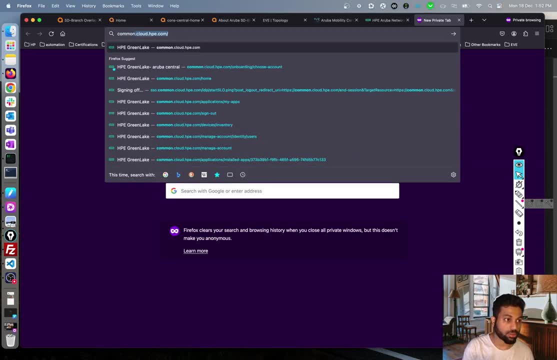 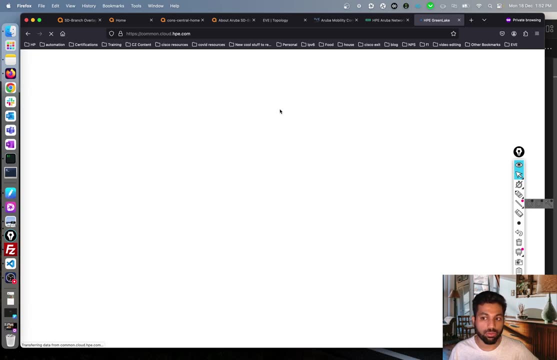 so i've got my browser here right. so let's go to aruba central so you can access it using common dot cloudhpcom, right? and then you need to put in your- you know- username and password. now, coming to aruba central, you might ask me, joel, how do i get access to aruba central right now, if you just 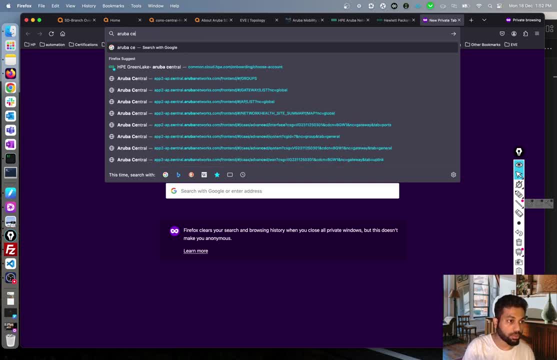 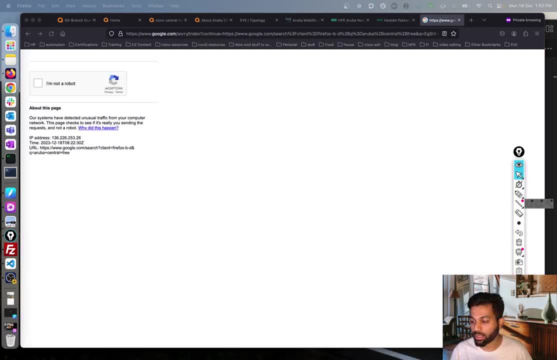 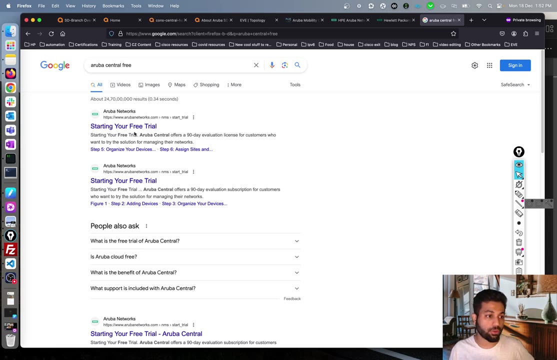 go and google aruba central, um, you know, free, right you will. you will find: uh, okay, that's one sec, all right, i don't know why google thought i was a robot, but anyway. so if you um just google for aruba central, free you'll, you'll probably find um. you know multiple links here telling you about. 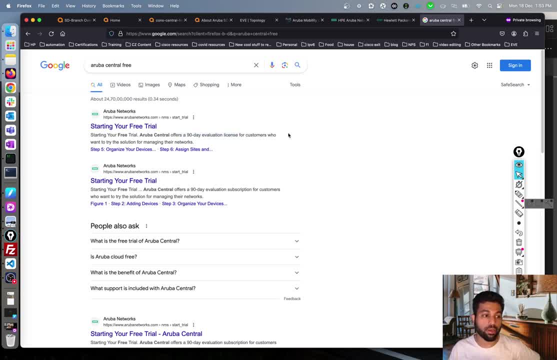 a 90-day evaluation license right for customers who want to explore um. you know aruba central so you can check out the check out how to get it right. so you should be mostly able to get a free aruba central for about 90 days. um, if you're not able to avail this, you know i would again suggest. 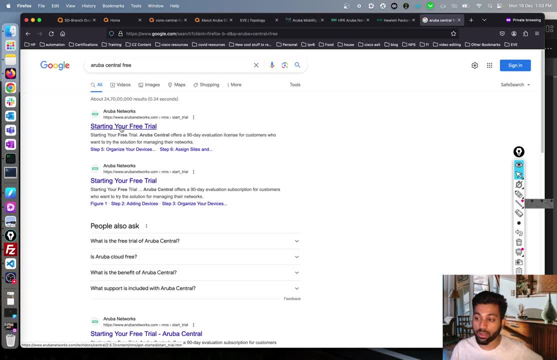 you to reach out to your aruba partners- or you know your aruba account managers- and they should be able to help you kind of get this so that you can explore the technology and get your hands on right. once you're done with that, you know you will basically get something like this. that's why 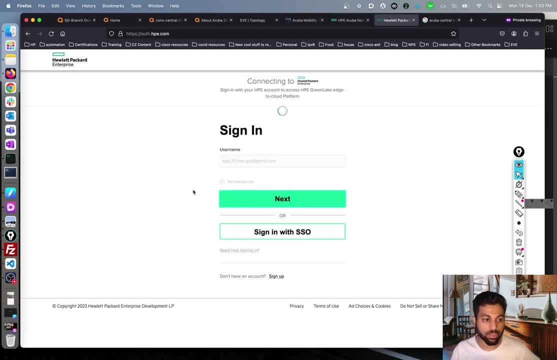 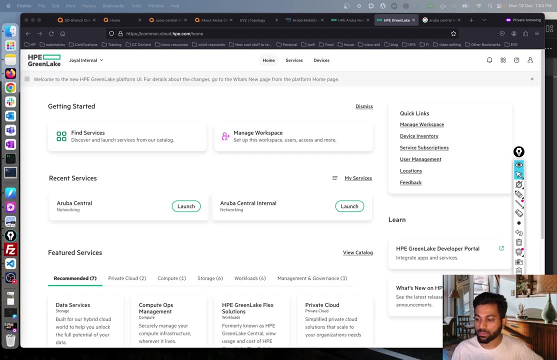 i'm using my personal email here and i'm gonna, you know, sign in. right, you can. you'll be able to create an account and sign in. let's put my password here and once you sign in, uh, what you get is something like this: all right, so this is the view which you get, uh, with aruba central, you. 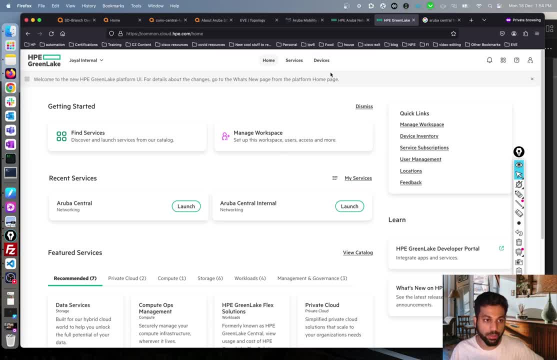 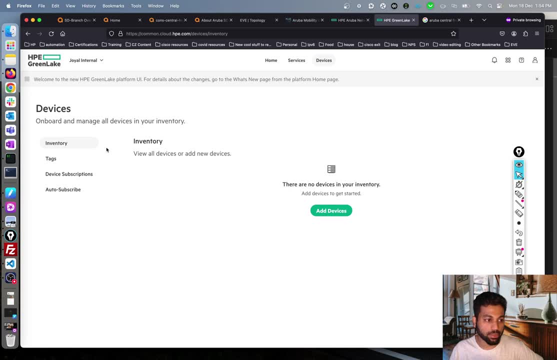 have a lot of things. for example, you can uh like for this particular account. right, this is the. this is just my lab account, i'm just playing around with it so you can see. um, you know, if you go to the devices, you will actually see the subscriptions and so on. um, when you, when you, 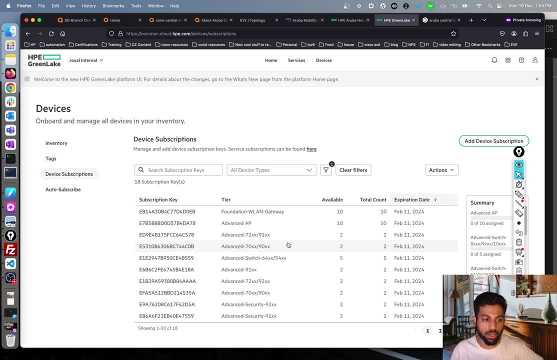 create a um- you know, evaluation um account. you should get some, a few subscriptions for free, right, maybe? like very, very small quantity, like two devices, five devices and so on, just for you to explore the technology again regarding this. if you don't have this, reach out to your you know. 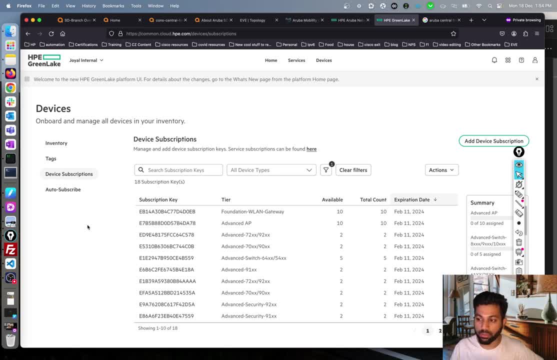 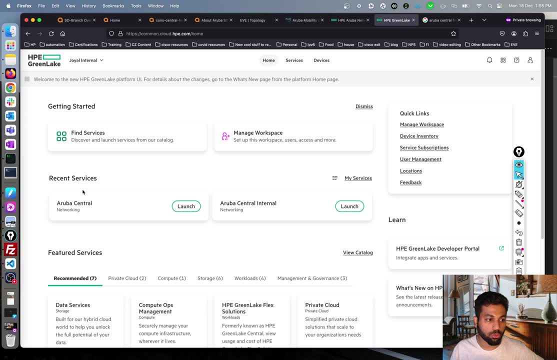 they might be able to kind of help you with getting you up to speed, to kind of explore the technology, right. but that being said, let's go to the aruba central platform, which which is over here, right, you, you, you will generally find there are a lot of other applications, you know which? 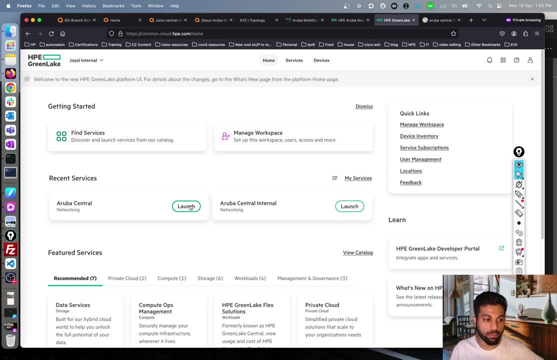 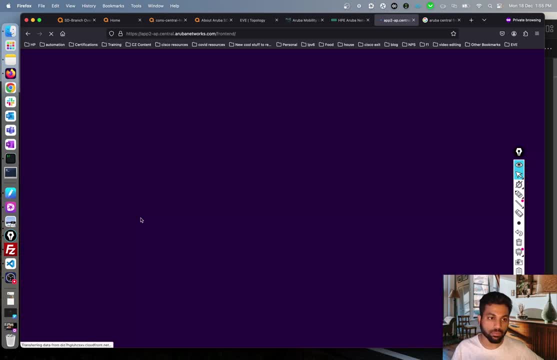 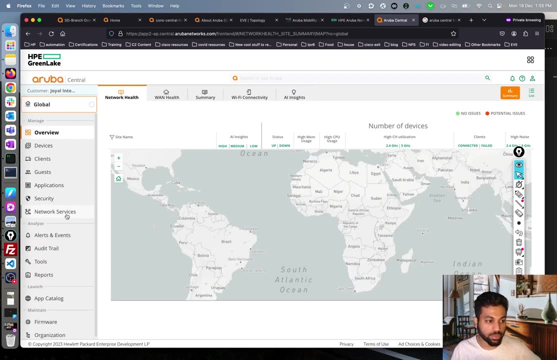 you can use inside the hp ecosystem, but the main one which we are interested is the central. so i'm going to go to central. so once you open up central, you get something like this right: perfect. so here all you need to do is come to this section. 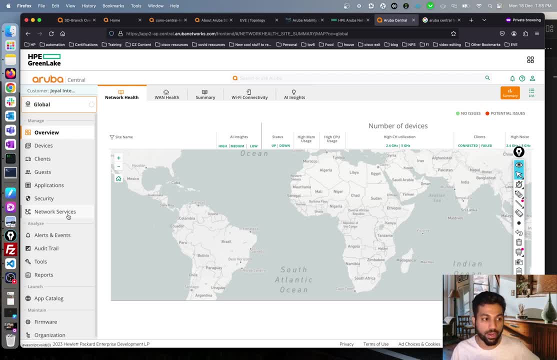 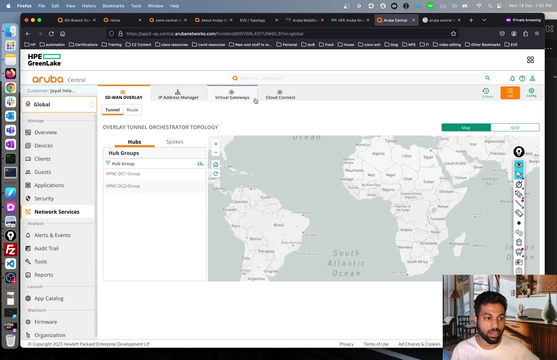 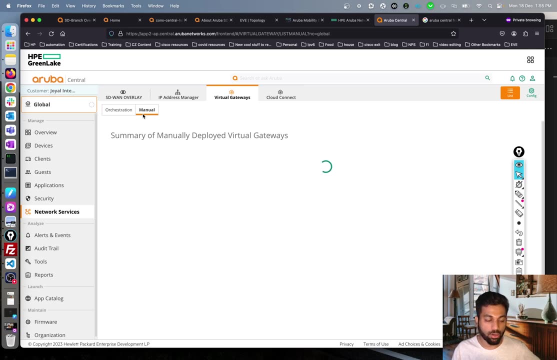 so right now, um, i have cleared out all my um, you know sites and groups and everything whatever is there in central. so it's completely blank. i'm going to go to network services over here, right, and go to virtual gateways, right, go to manual and over here i can generate those ioso files. 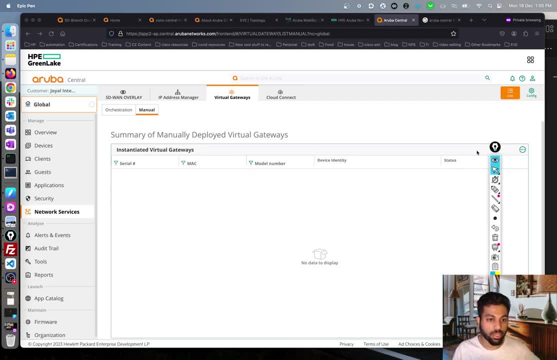 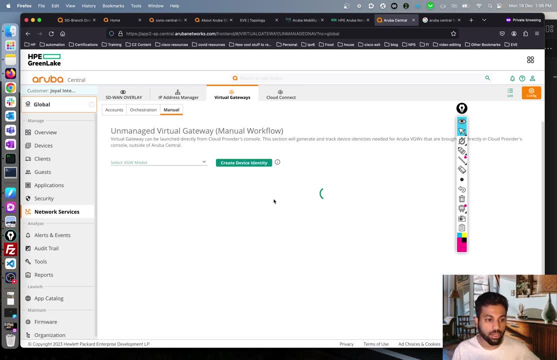 which i talked about, right? so here, uh you can see, right now there is uh nothing, right? so i'm going to go to config here on the top right, right, and go to manual again, and here you can see, these are some of the so i have. uh, you know, i'm allowed to create four gateways, right? 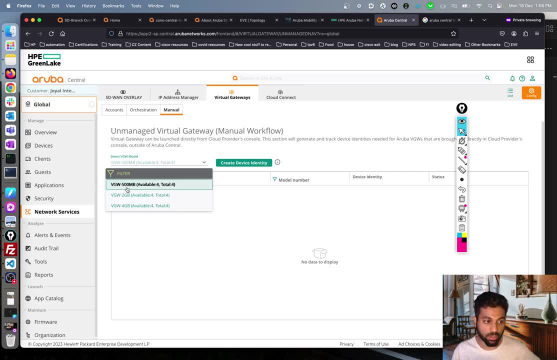 i can create four gateways, uh of each types. right again for for the lab purpose. i can use just the, because i don't think i'll be even sending 500 mbps. but again you have different uh virtual gateways based on you know the throughput which they can give you, like two gig, four gig and so on. 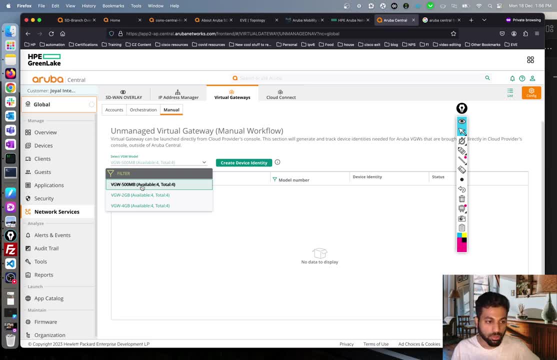 any of those, but i'll be using just the 500 mb ones. so i'm going to select it and i'm going to say create device identity and it's going to ask you. i'm going to say yes, right. so there you go. so it created. it's going to take a few seconds. right now it's in the init state. let's come back after. 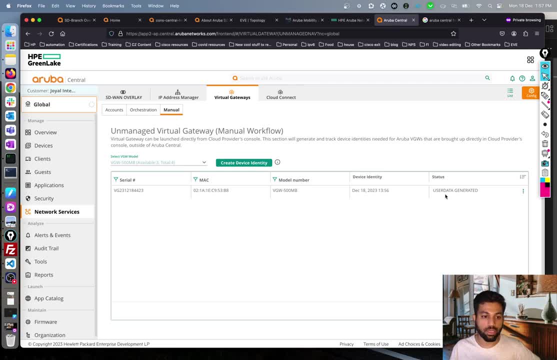 probably a minute, perfect. so once it is generated- now you see, you get something like this user data generated, right, all you have to do is go here and click download iso. so once you have that iso file, next what you need to do you need to upload this iso file to your evng. you know vm. so what i'll do: 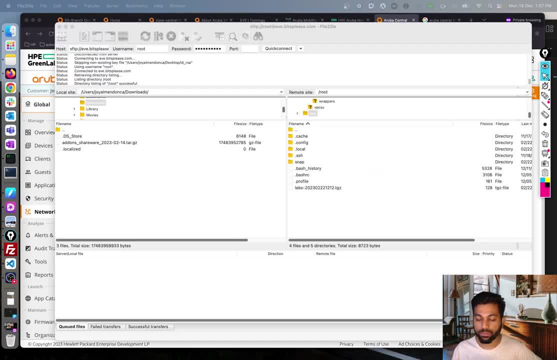 is, let me do that. there you go. so i've pulled up my- you know- file zilla where i'll be uploading this so that i can show it to you. right, let's go to the location. which location? so i'm going to go to opt unilet, add-ons, chemo and inside chemo. 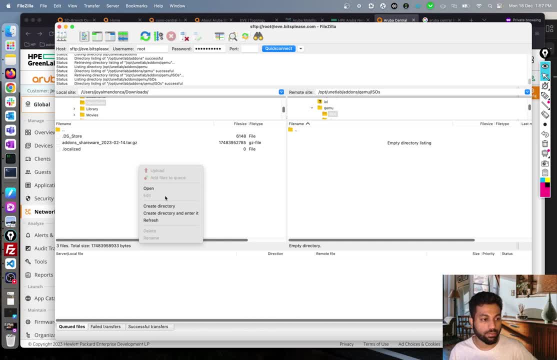 i'll be uploading this so that i can show it to you. right, let's go to the location. which location created a separate folder for isos? and here, from the reference side, let's refresh it. so there you go. that's the file i downloaded. i'm just going to upload it. right, and the file is already uploaded. 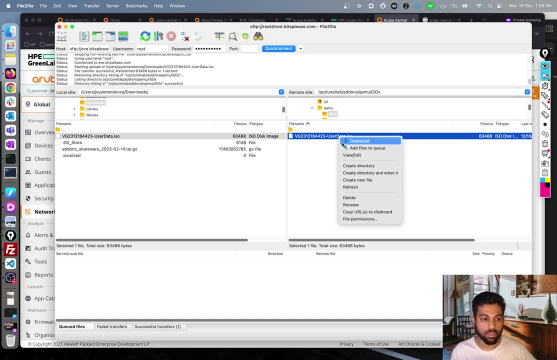 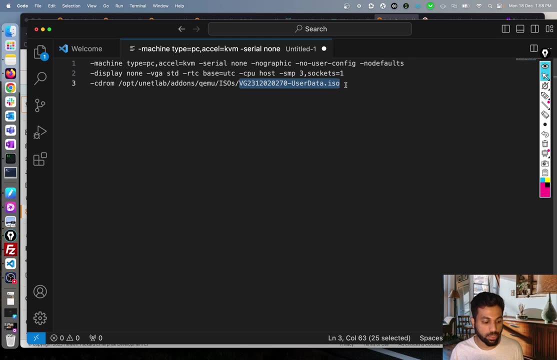 so, now that, once you have that, all you need to do is, right, copy the name of the file. in this case, i'm just going to copy it from here. right, let's go to that, you know, let's go to our- you know- text editor. what i'm going to do now is just replace this with: 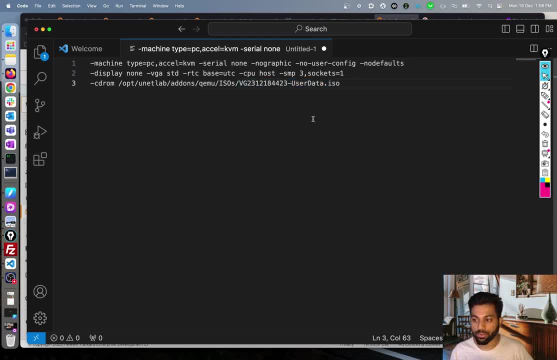 the name of the file, right? the ios file which i generated, and now you just need to copy the whole thing, right? let's actually make sure that this is in the same line, so i'm gonna send it to the same line, right? there you go. now i'm going to copy the whole thing. ctrl c and let's go to our 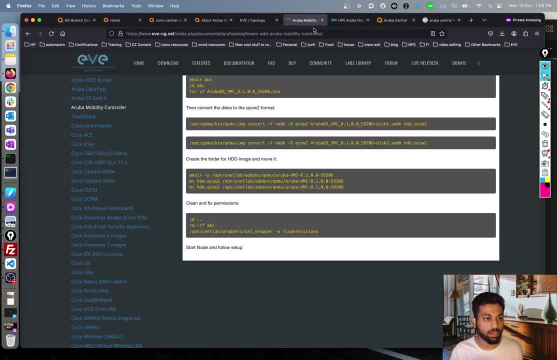 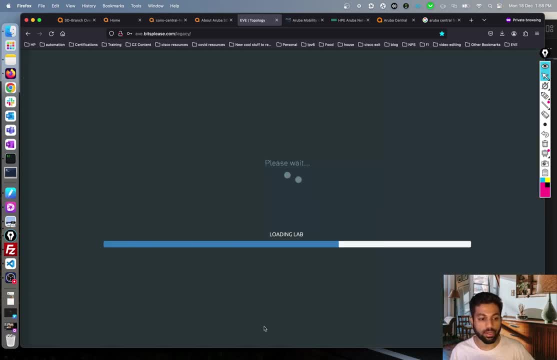 let's go to our evng over here. where is our evng over here? right, you just need to replace it over here, paste it. that's it, right. paste it, save it, and then you know, one of the devices that i'm going to create is going to be Wasp. gets the same configuration as the others and you can see that the device is. 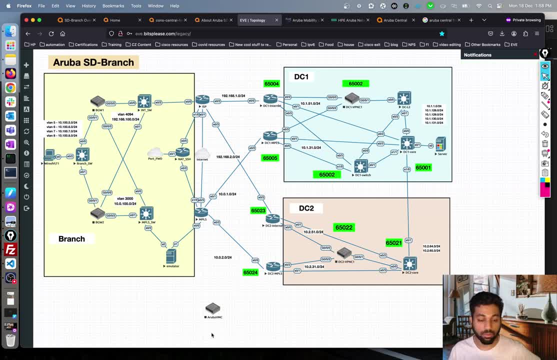 up. that's it, i mean, that's all. that's all is needed for you to get the device up right so that you but you need to generate separate iso files for each of your devices. obviously, whatever i showed you was for one device, but for the second device, again, you have to do the same process, go and. 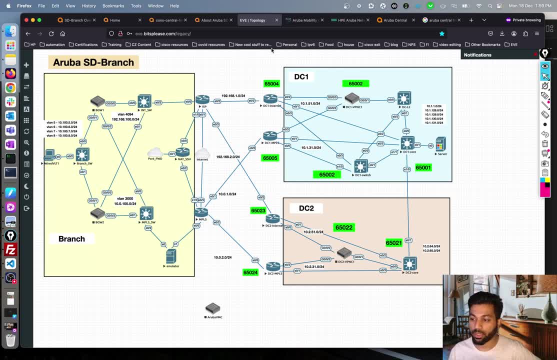 generate the second iso device iso file, put it into your evng and you know um update the chemo options on that device. so i i will be doing that for all the four devices showed you for one of the device, right? so yeah, that's everything which i wanted to show you. 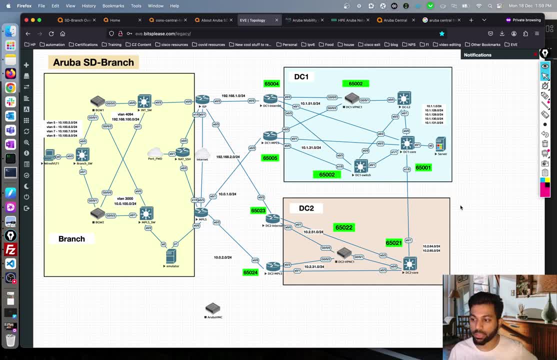 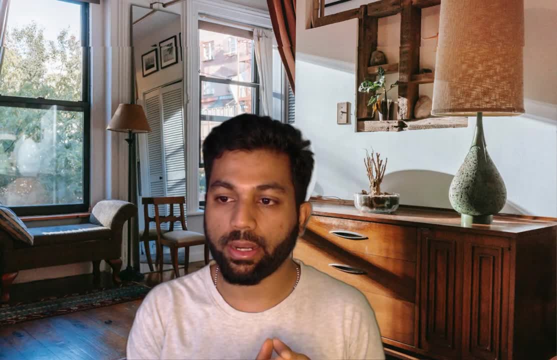 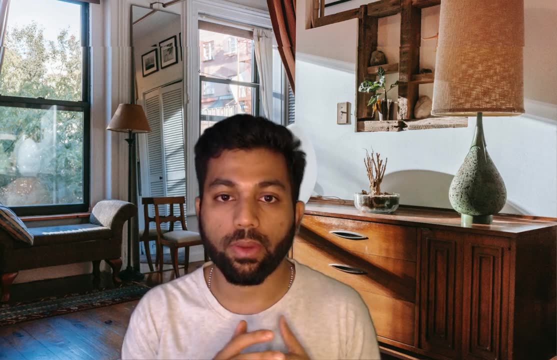 before we start with the actual hands-on in the next video, right? so just to recap, what did we do today? we kind of started with getting a quick overview of the solution, right. what aruba st branch is all about? what? what are the various components, what are the various topologies? you? 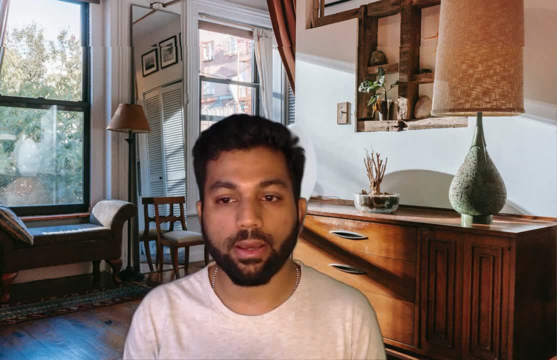 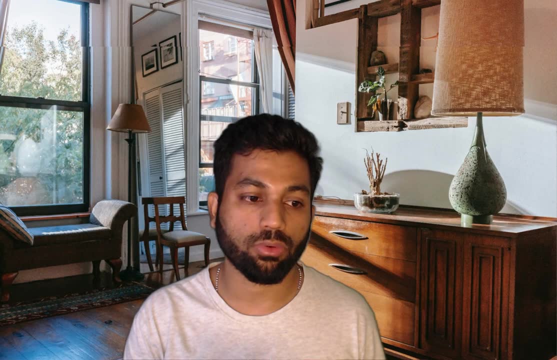 create with it, what are the various types of policies and so on. then we looked at our lab. we try to understand how this lab is set up, what are some of the prerequisites, what are some of my learnings which you can use to kind of, you know, bring up the lab quickly. so, yeah, i think, hope. 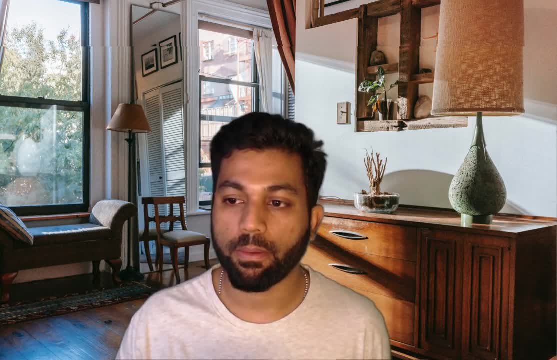 that was useful. do come back on the next video where we'll be discussing more on some of the actual hands-on exercises. okay, ciao, bye.